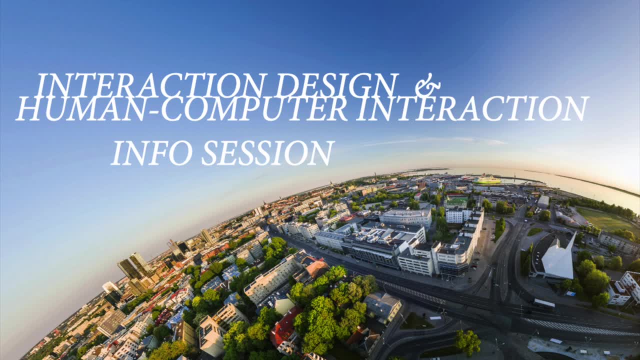 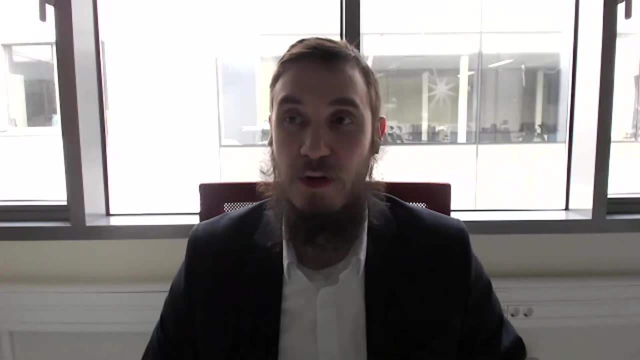 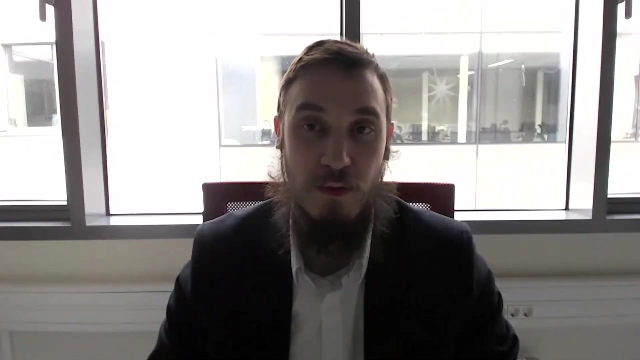 So my name is Ilya, I'm the head of the Human-Computer Interaction Study Program at Tallinn University, and together here is also my colleague Sonia, who will do the introduction for Interaction Design, and also Andreas, so both of them are managing the Interaction Design Master's Program, and also our students Gabriela and Sean, who will give you a little brief introduction. 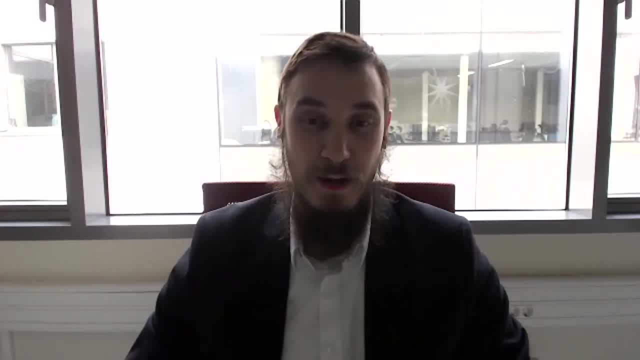 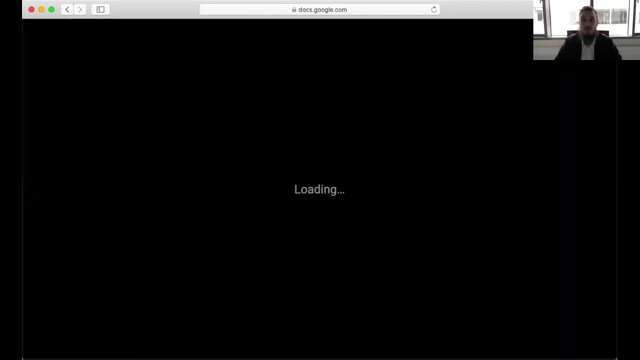 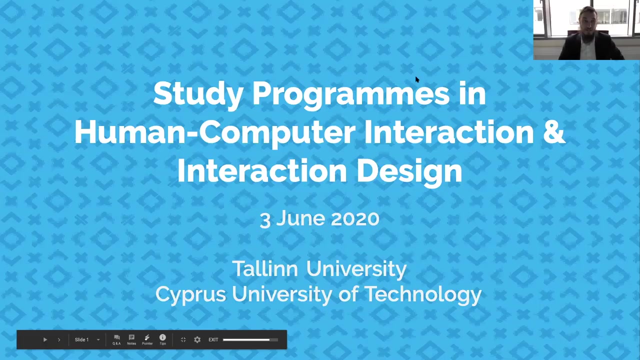 Okay, so I'll try to share my screen now and we'll go through the presentation. So I hope everything works nicely. I'll try to go full screen so that everyone can see. Okay, so I hope that you can see the slides. If not, please let me know. but I really hope everything is working. 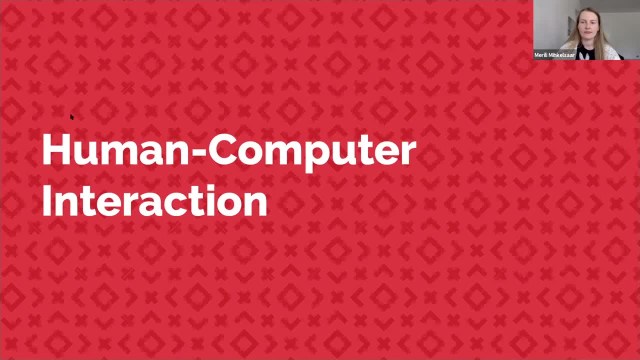 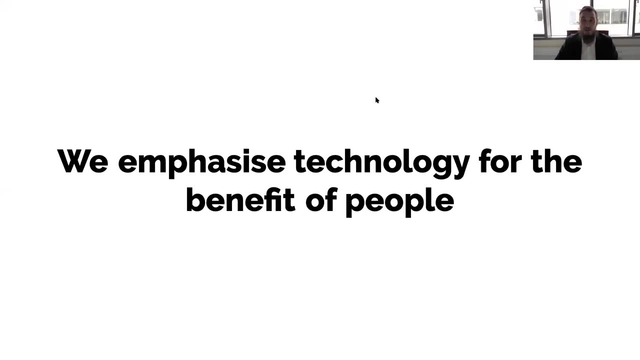 And briefly to introduce the HCI Study Program to you. So in the Human-Computer Interaction Study Program we emphasize technology for the benefit of people. That's our kind of tagline, that's our model and that's how we try to also. 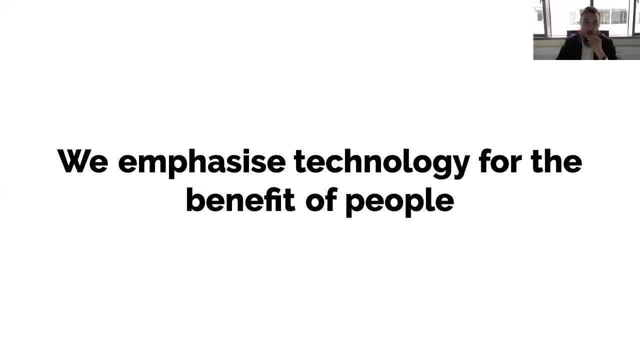 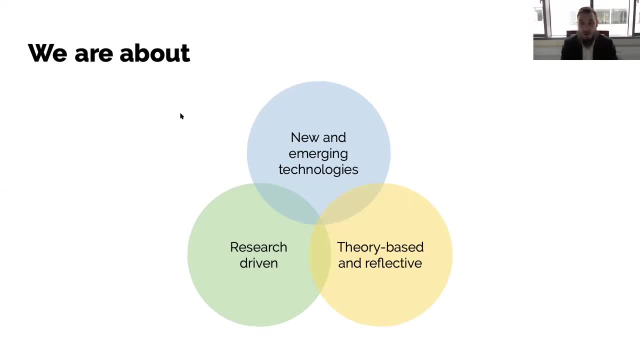 approach things on a day-to-day basis. What are we about? We focus on three main things. One is that our Master's program is very much research-driven. It's informed by our latest state-of-the-art research that we do within our group. 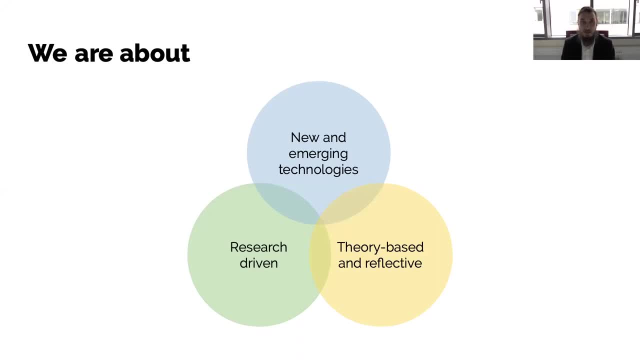 And that's why, also, most of our teachings, most of the lectures, most of the classes that were organized, most of the material that we share with our students, is not from the book. It's from our ongoing state-of-the-art research. 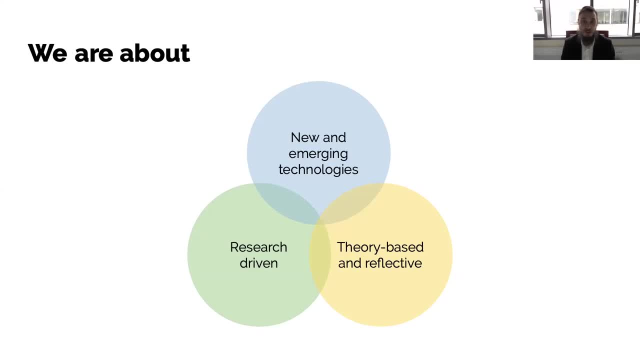 That's something you cannot go through with, something that's different from what you're doing at the moment. go to a library and read about. that's something that we share with you. on our fresh experience, we focus on new and emerging technologies, so we like to. 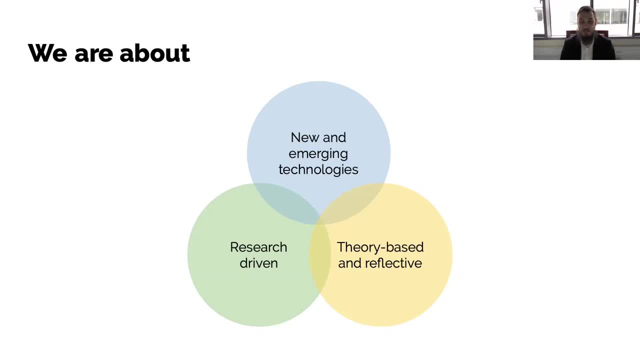 think of ourselves as working on things that will only become commercially available or mainstream in five to ten years. so that's also kind of one of the our focus areas. that's what we try to to to play with technologies that will only go mainstream in the future, and we're also very much theory based and 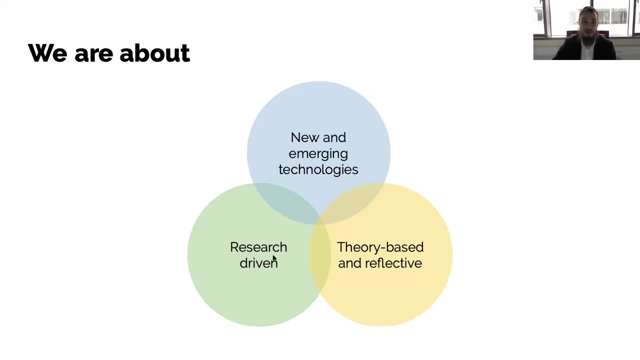 reflective, which again I guess feeds back to this research driven approach. so most of the discourse that we have in the various sessions, in the various modules, is based on theory. we, when we engage in hands-on activities, in the design process, we'd like to be very much reflective and critical about what we. 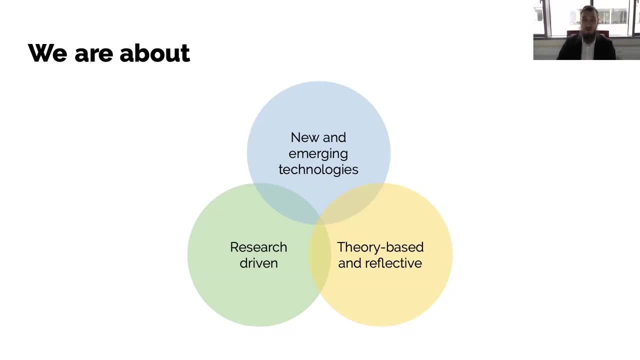 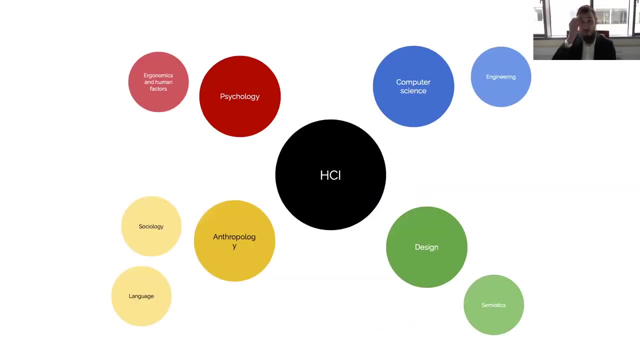 do and how we put together and what values we use. so you, I think it kind of these three things, these three facets, permit very much what we do in the program. if we look into the background of the students that you might eventually encounter in the program, then it's very diverse because 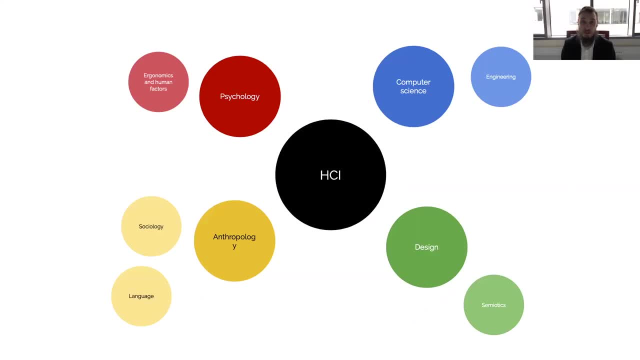 the. the field of HCI is also very diverse, so I try to point out four main areas of where people come from to study with us. it's mainly computer science, design, psychology and anthropology, but there are also kind of surrounding disciplines such as economics and human factors, sociology, language, semiotics, engineering. so it's a very mixed crowd. 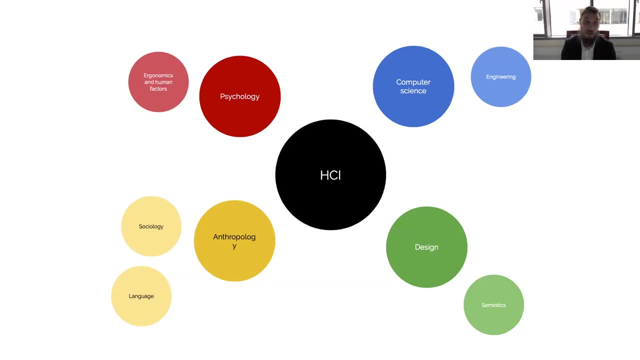 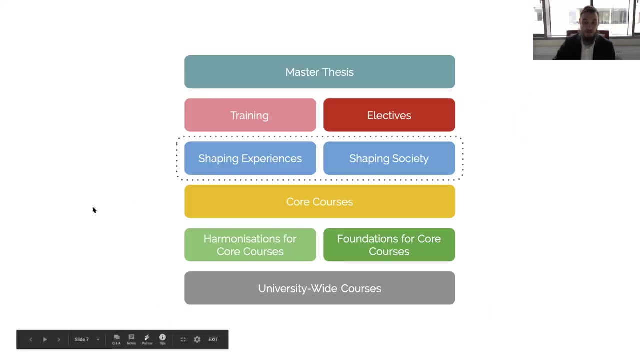 of people, some with more engineering or more technical background, some more the more artistic or design based background, some from social or behavior sciences. so different understandings, different schools of thought, different approaches to design, research and technical implementation, and we put all of the new and all of them together to make cool stuff happen. let's see. oops, sorry. 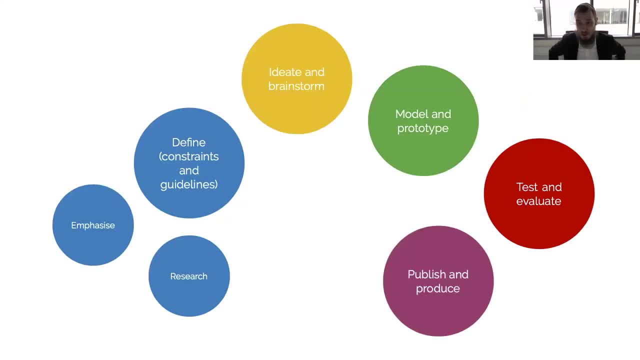 so how are our studies organized? how would they go about approaching things? well, we go through several stages of. there are several different types of activities, from emphasizing and researching to defining the problem statement through constraints and guidelines, and then ideation and brain storming, and then modeling and prototyping, testing and evaluating. 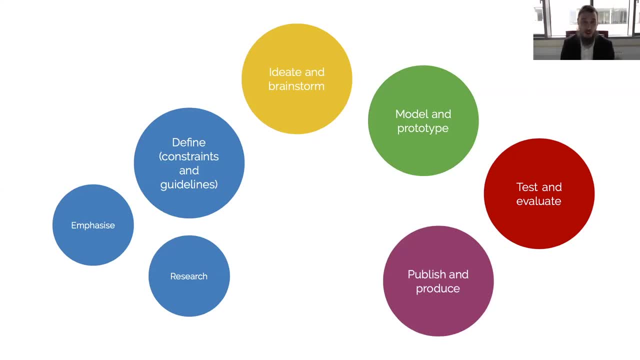 finally publishing and producing. so in the course of the studies, you would cover the whole range from from contextual inquiry and background research to creating or defining the design challenge or the problem statement and finding solutions, exploring alternatives, how to implement things and then evaluating with users, assessing and finally producing the 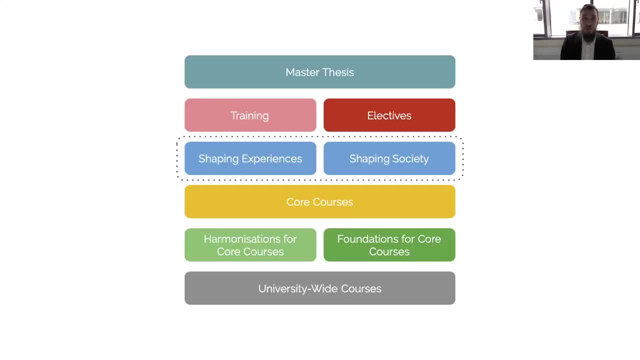 final outcome. the course overall the program is is a two year program, four semesters, and this is how it's mainly structured in the main category. so if some of you have already looked into the more formal program description and you might see that we start with university-wide courses, which is like a foundation, and 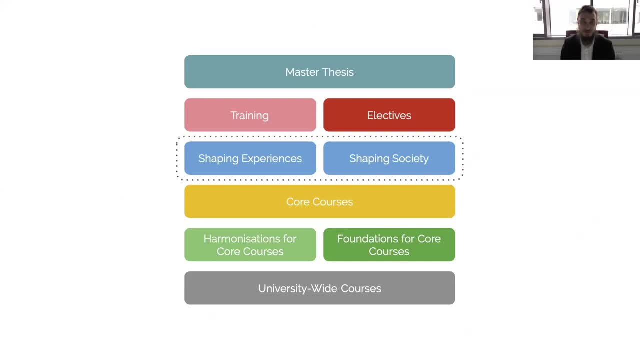 the course that we have. there is them is the interdisciplinary course that we run throughout the the university. so all of these courses are really based on the. you can interact with people from all sorts of backgrounds and programs from all the university, and then there's a set of harmonization courses. so 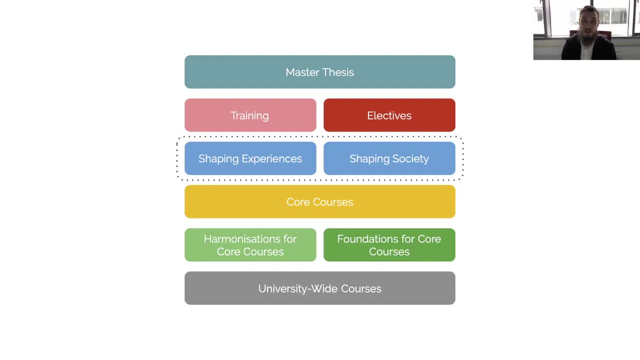 depending on which background you come from- either design or technical background, or maybe social behavior sciences- we will look into what skills you're missing- either design or programming, development or both- and then you get the chance to get those skills. and also there's an intensive foundations section which teaches you a lot about the theoretical landscape of 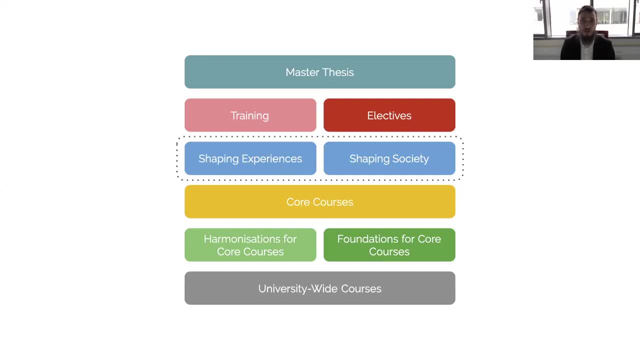 HCI, the different research methods that we use and how to go putting together your initial research proposal for your master thesis. then there's a set of core courses and then tool selection modules, either on shaping experiences or shaping society, depending on which way you want to go, either focusing on the micro or 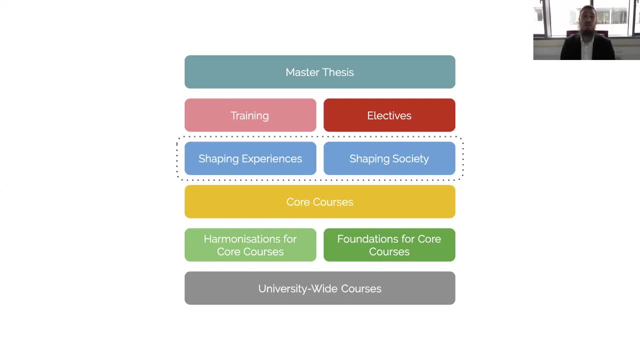 the macro level of designing interactions. and then there's training, either through internship or training abroad, and a set of electives, that where you can choose from a set of different courses that will offer to kind of create your own unique profile and path, and then, finally, we wrap off the course with a master thesis project. 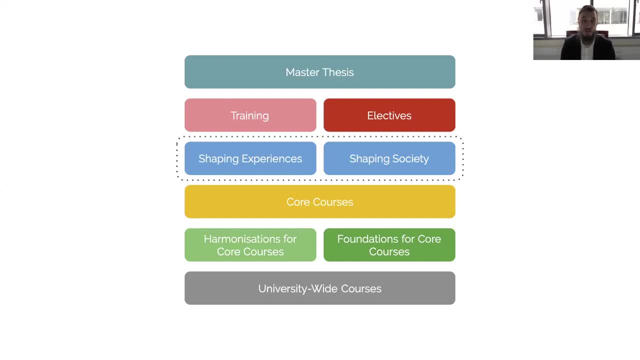 which is kind of project you work on on a selected topic with your supervisor to build very nuanced and detailed expertise in a certain area, that of your interest. so on the next slide, as soon as it opens, you will see the breakdown of the different courses throughout, throughout the semesters. so, like I mentioned the, the program is a. 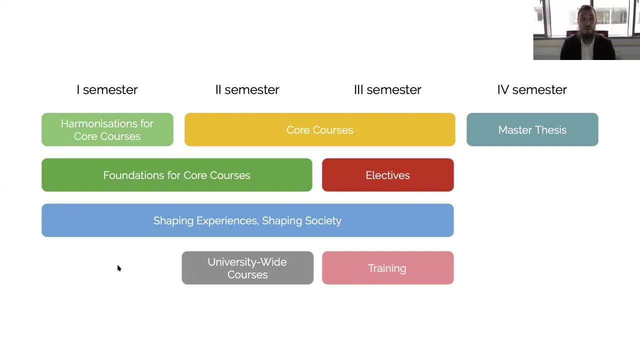 four semester long, two-year course. in the first semester we start with this harmonization, or we call them up to kind of getting your skills up to date, basically courses. then there's a set of foundational courses which last for the first year. core courses are the core. 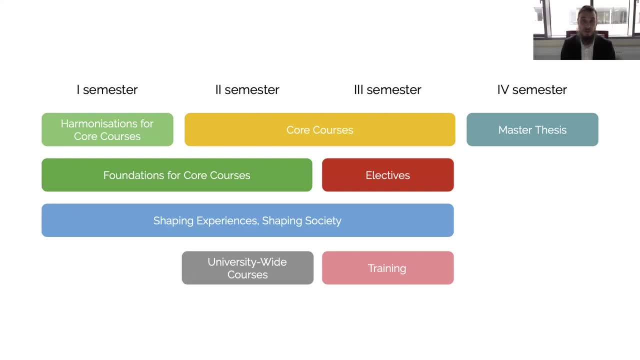 courses to the HCI curriculum, mainly focusing on the foundations of HCI, and also this shaping experiences, shaping society module, which is kind of you can choose which path you want to go through. in the second semester you also take these university-wide courses, and then the third semester is what we call our mobility window. so it's either you take a set of selectives, 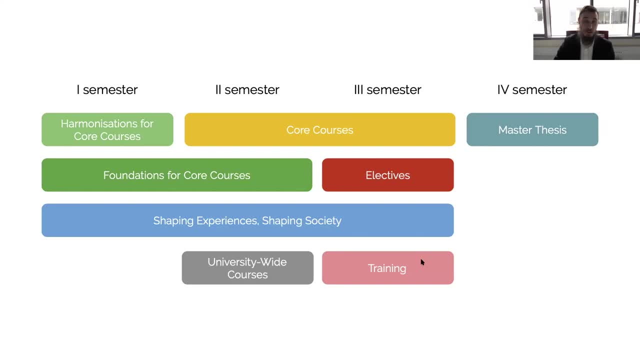 or you actually can choose to go abroad on an Erasmus exchange to study in a in a different university in different country, and the fourth semester is actually devoted to the master thesis. so this is roughly how you your studies could pan out over the four semesters and you can. 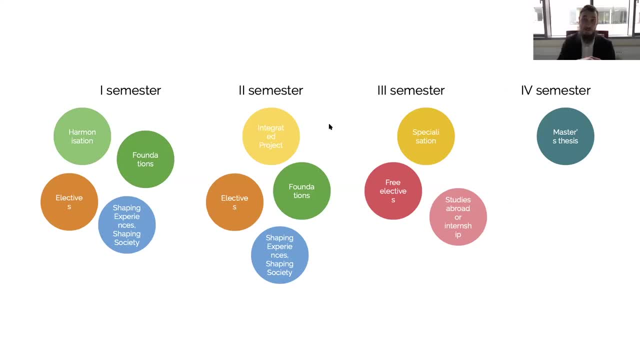 see here a more detailed view of how these courses are organized, similar to what I was showing to you before. so there's foundations, harmonization, shaping experiences and society, based on two or three objectives that you can take in the first semester. in the second semester, we mainly focus on an integrated project, which is a very hands-on activity. 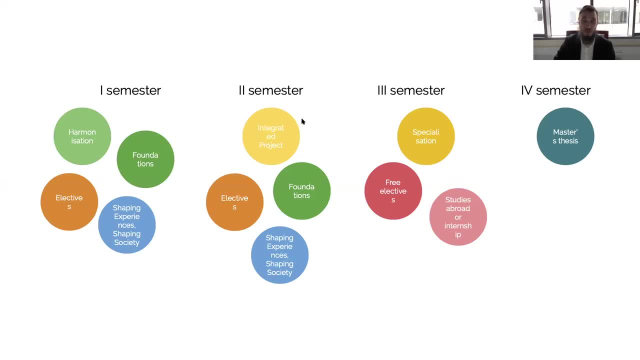 which where you go exactly through this process of coming up with a design challenge or research in the background and then finishing off with the working prototype that has been thoroughly tested with users. finally, in the third semester, you go for this kind of studies abroad or internship in a company, free electives, and then you finish off with the master thesis. 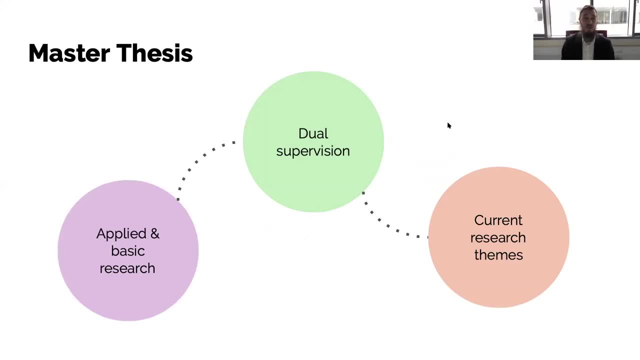 okay, so, to tell you more about the master thesis, because we're going to talk about three of these things, of course, we're going to start with the master thesis and then we're going to talk about the first one, which is the project that we're actually really into, because we're 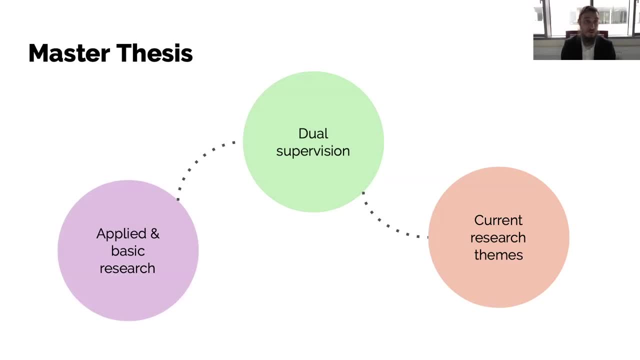 that's again related to this research driven part of our studies. We try to go for either applied or basic research, so you can do a hands-on project developing or designing something, or you can actually go for basic research and go maybe more into theory building and creating. 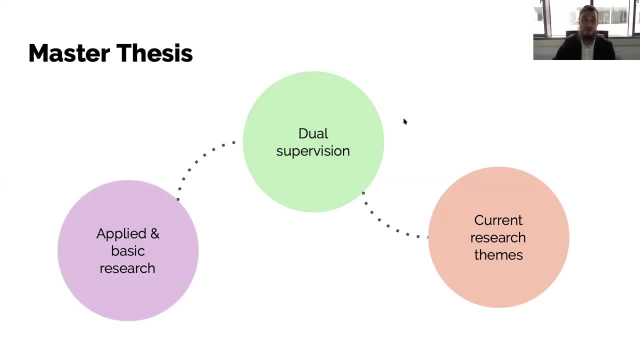 different models. We usually go for a dual supervision model because we try to go for thesis topics that are very much multidisciplinary, so bringing in or combining several different areas of expertise, And we frame them within our current research things, which are four, I won't 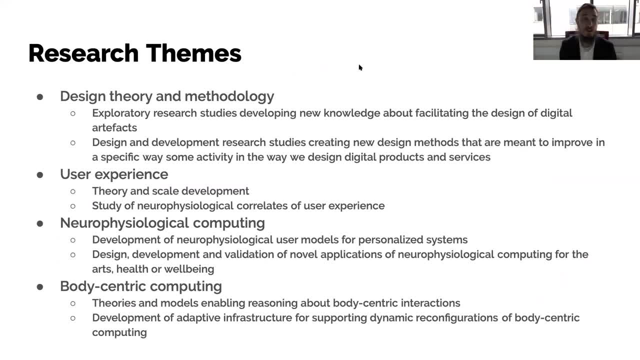 go through too much detail on that. We have these topics also posted on our website, But we work across four main areas: Design, theory and methodology, user experience, neurophysiology and body-centric computing. So some of these are overlapping and combined, And then there are a few that are still there, so we try to go through them. 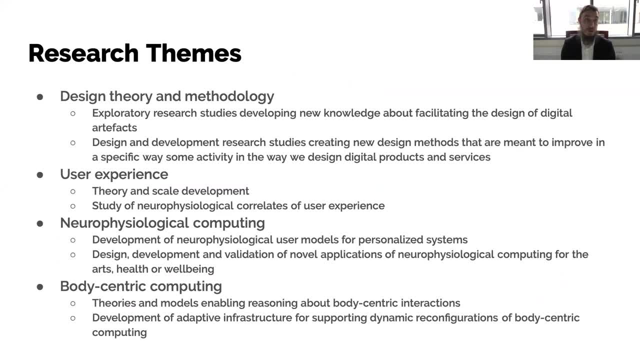 complementary and, depending on where your heart lies closer to the most, you can choose and position yourself within one of these topics, and what you can see here on the slide are some subtopics that kind of try to illustrate what this work within one of these larger areas could be about. so all of our students, 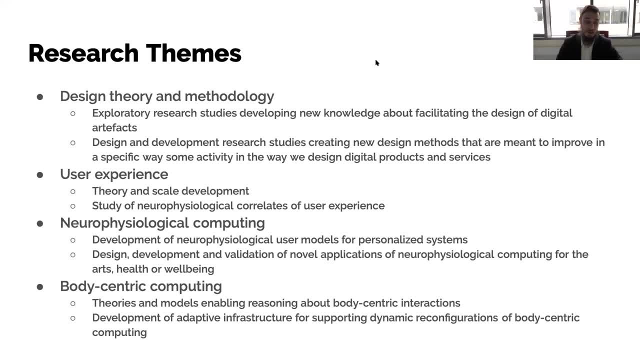 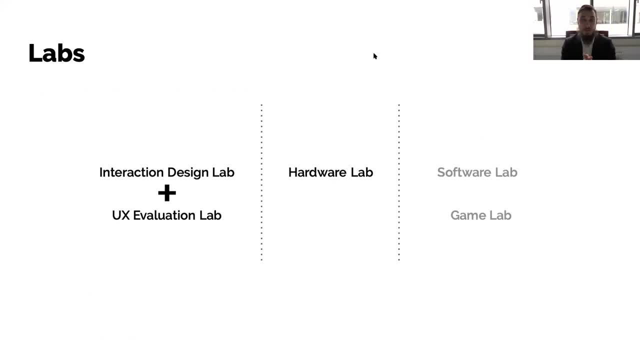 eventually need to position themselves and their master thesis within this, within these four topics, or within one of these four topics. okay, so we also have a very nice infrastructure to support our activities. we have in our school, in our Institute, we have five labs, but we're mainly using the first. 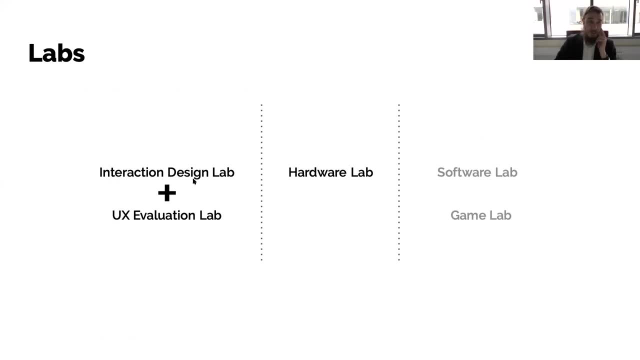 three ones. most of our activities are based in the interaction design lab, where we go into kind of this. we have a space, an open space, which kind of facilitates all the activities within the four topics, within one of these different conceptualization and prototyping activities. and then there's 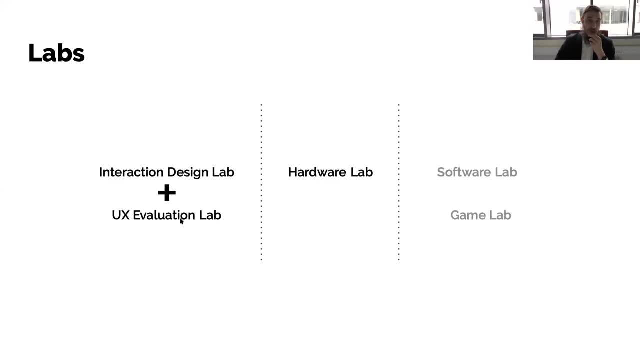 a companion, smaller lab to it where we run controlled lab experience using different equipment that I'll show you in a moment. and then we also use the Haru lab, where we mainly go into body centric and yep own-body computing. we also have the software lab and game lab, which also 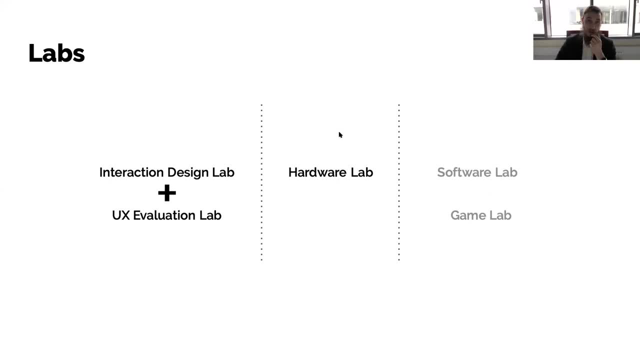 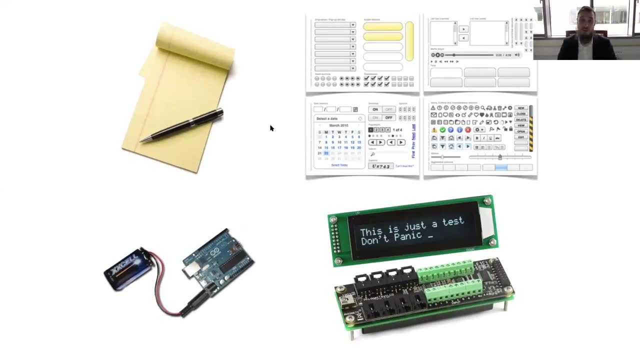 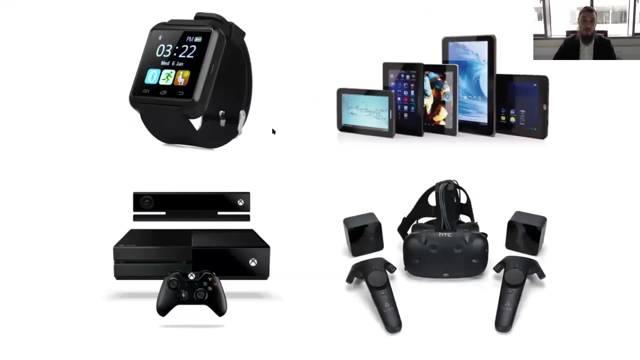 some of our students use, but mainly these three ones that I kind of highlighted here. Okay, so some of the tools that we use: we go from paper-based to very hands-on: microcontroller and electronics materials. We go and explore different types of devices and different types of modalities from wearables. 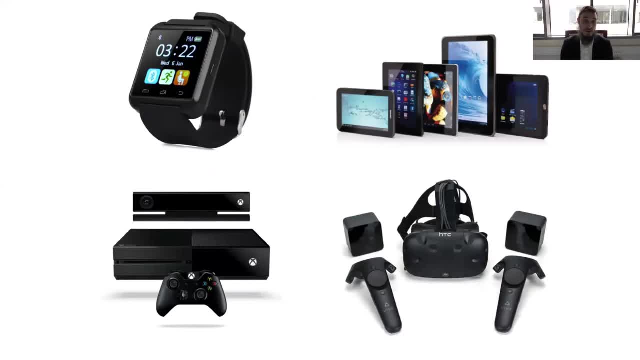 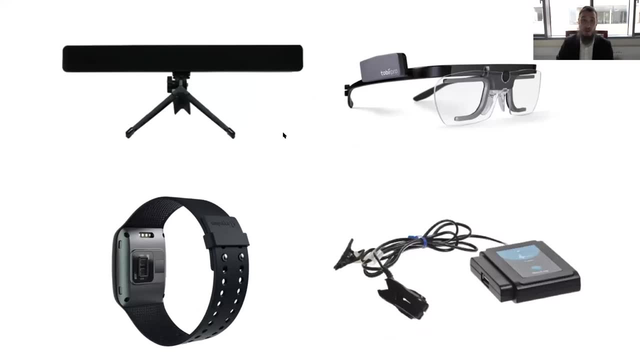 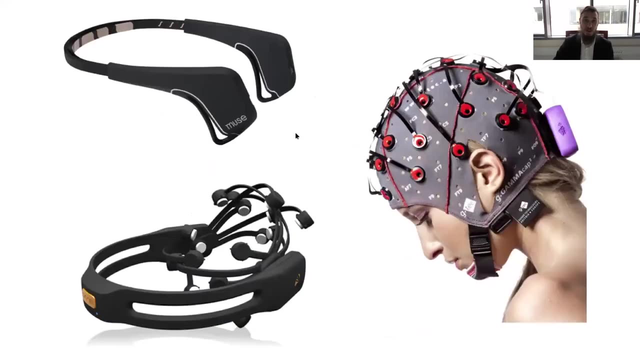 to virtual reality, to touch screens, to motion sensors and game-based interactions, to physiological computing such as eye tracking, emotions, emotional state tracking, to finally tapping into your brain and actually looking into how your brain reacts to certain things, reacts to stimuli, reacts to interactions that are being kind of designed, and also how you can. 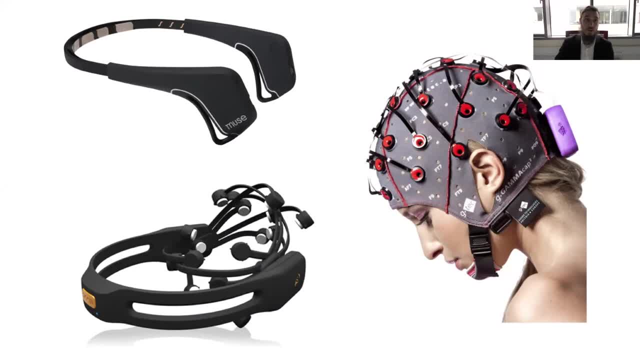 interact with the system through your brain, So kind of this goes both ways. So, as you can see, a whole range of different materials And devices and equipment that we use. all of this is available in the labs that I mentioned to you before. 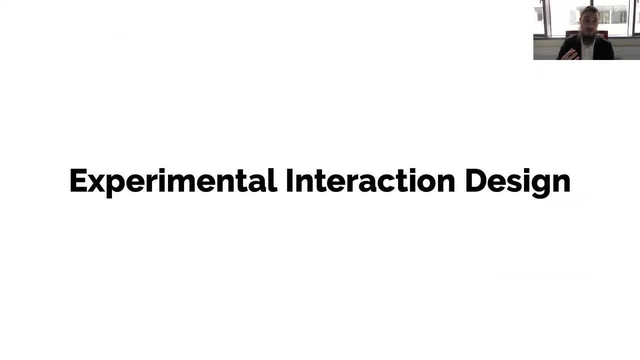 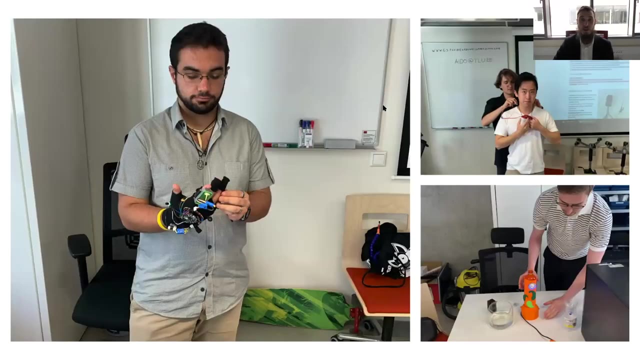 And finally, we also have different kind of tasters or flavors of our of the courses that we teach in the program in different formats. One of them, the most maybe the oldest one or the more mature one- is the Experimental Interaction Design course, where we actually go into a two-week intensive process of conceptualizing. 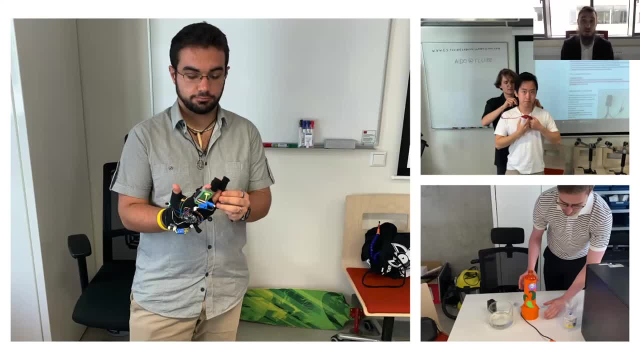 designing and prototyping body-centric interactions- And this is just some examples, with students coming with necessarily no design or development background and, in two weeks, building working prototypes with Arduinos and microcontrollers. So this is just a glimpse of what we're doing in just two weeks. 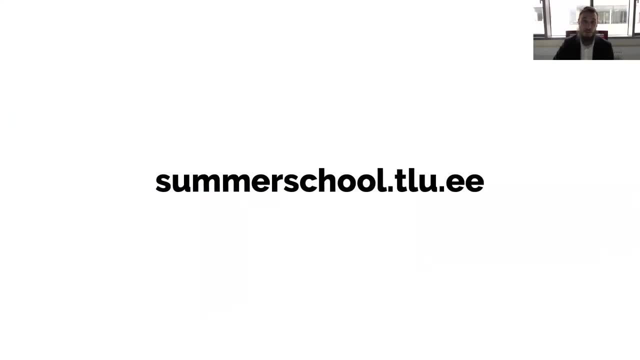 You can read more about it either on the summer school or winter school variant, because we run this course twice a year. We also run the annual World Usability Day event, which I think the last couple of weeks- I think the last edition it happened- took place on November 22 in the Talent Creative. 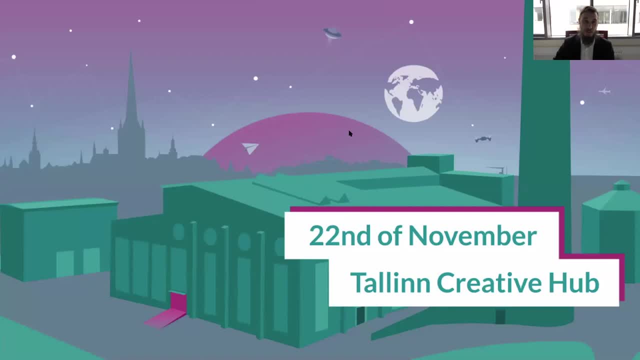 Hub And it brought together around 500 people from the Baltics and the neighboring countries, such as Finland, Russia, Sweden. People come from all the region to join for this one-day full event of conferences and presentations and also an accompanying two or three days of presentations. 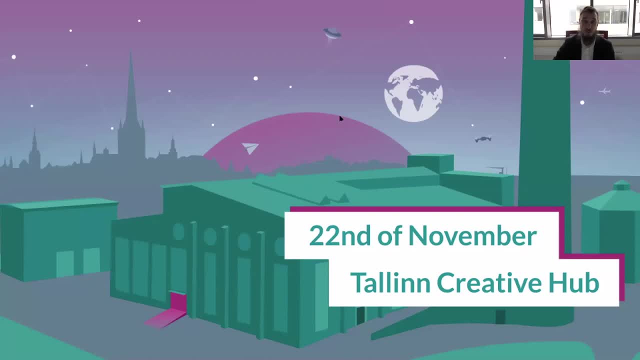 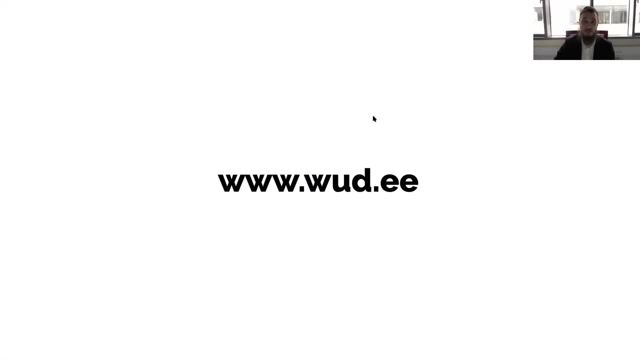 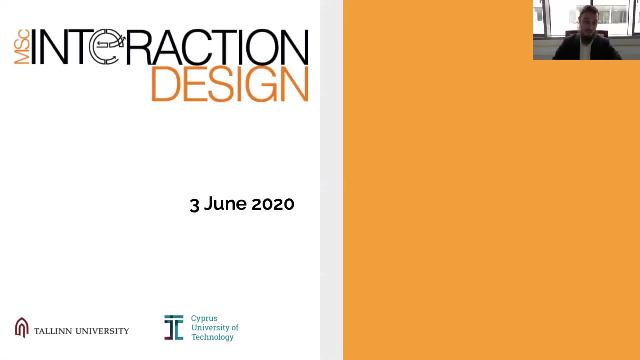 So this is kind of also a very big event that we're hosting every year. You can read more about this here on the website wwwwoodee, wwwworldusabilitydayee, And I think that's it. That's what, briefly, I wanted to tell you about the program in exactly 15 minutes. 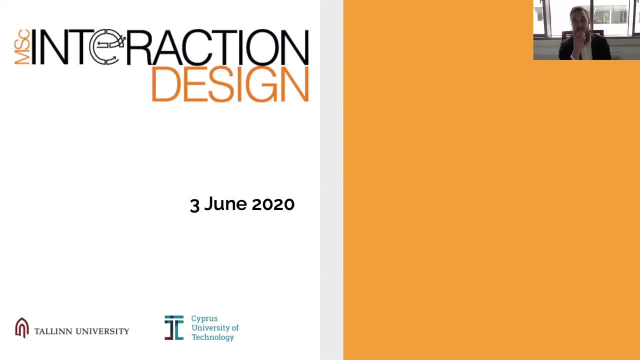 So I'm on time and I'll hand it over to Sonia and Andreas. Okay, Thank you, Ilya. Thank you, I would like to welcome everyone to the information session first And I will be introducing you the Interaction Design Master online. 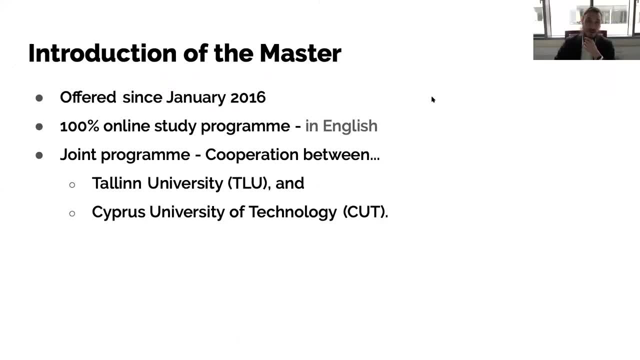 Can you go to the next slide please? Yeah, just tell me when to switch slides. So, basically, this master is offered since 2016.. It's 100% online study program. It's run in English. It's a joint program. 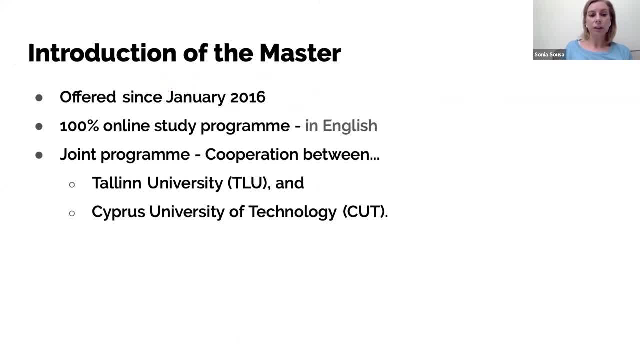 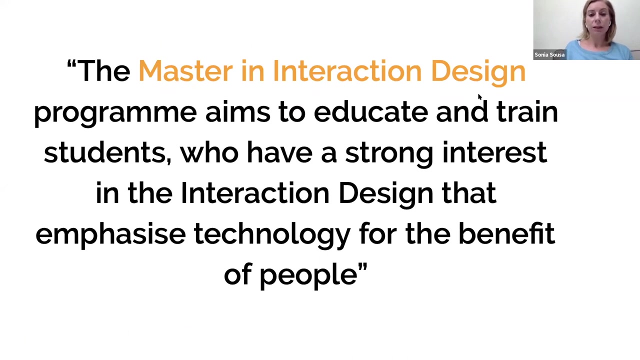 So it's run in cooperation between two universities: Tallinn Universities, where I'm the head of the program, and Cyprus University of Technology, where Andreas Papalis is the head of the program. So we have two heads. Thank you for this program. The aim of the master basically is similar to the HEI. master is to educate and train. 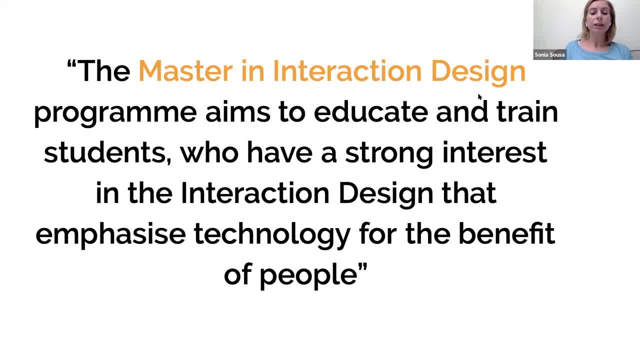 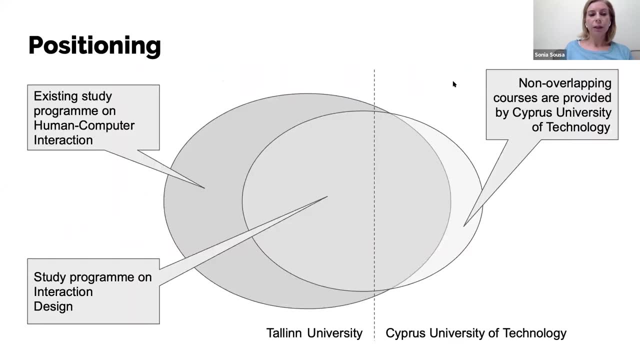 students who have a strong interest in interaction design. Also, we emphasize technology from the benefit of people. So, in terms of position, can you switch, please, Ilya, Positioning this master? it has been created from an existing program that is human-computer. 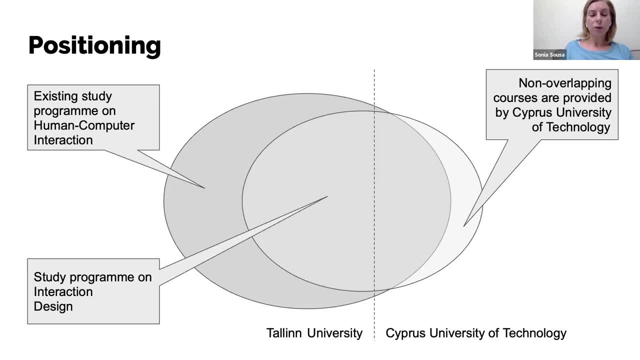 interaction And it overlaps. Okay, So you can see that it overlaps in this sense. And to that I'm not saying that a design is a memories program, It's more of a knowledge program And you can see that the courses are gathered from Cyprus University of technology. 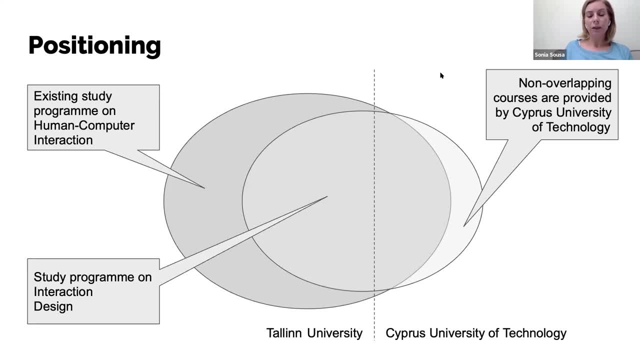 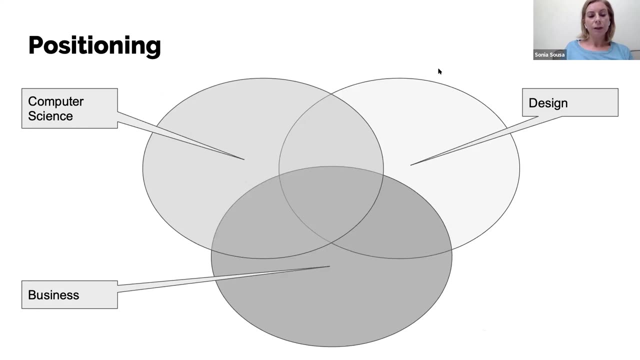 So you can see here that it kind of overlaps in this, in this sense the University and second in University and gains from this. both Universities experiences. The next one, please. So in terms of human interaction, fields and or areas, we, we, we prime the computer science, the business and the. 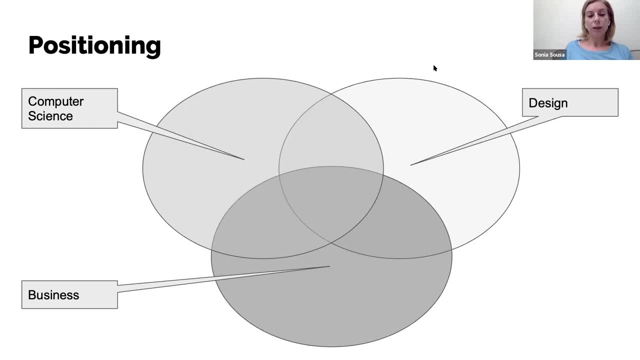 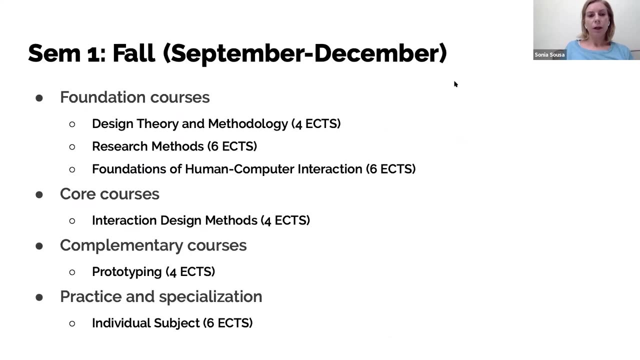 design area. so all of these overlap a little bit about the program. so in the it's the same as the HCI program. so four semesters to three years course. in the first semester for semester that runs from September until December, we have a set of foundation courses, core complementary courses and practice and 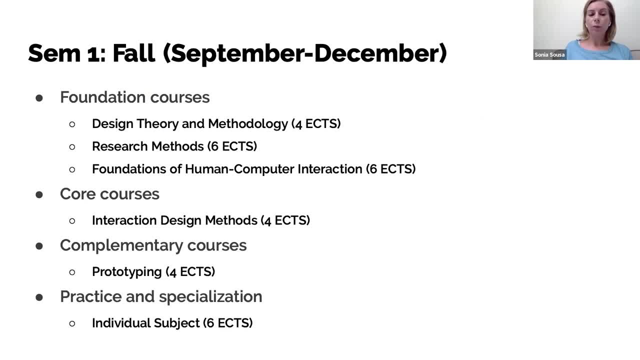 specialization that all of them are compulsory. so foundation courses are like courses like design, theory, methodology, research methods, foundations of human computing, interaction. the core courses are like courses like interaction, design methods, complement areas, prototyping and practice, and specialization is individual subjects, where we invite students to select a set of individual subjects to study that they would like. 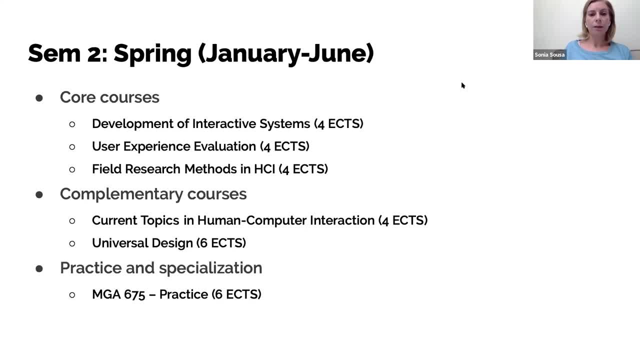 to complement in that program- the next during spring, from January to June- we also have some set of core courses, complementary courses and practice and specialization. so the core courses here are development of interactive systems, user experience, evaluation field, research methods in HCI. the complementary are current topics in human interaction input, human computer. 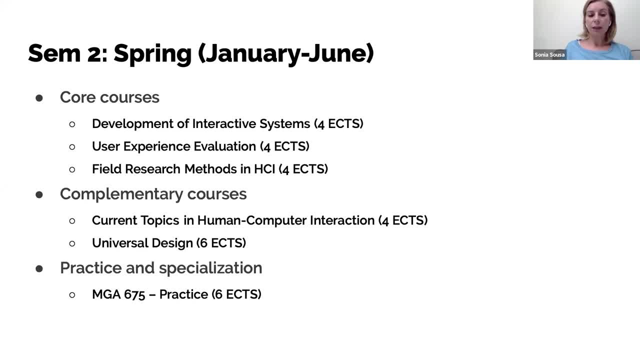 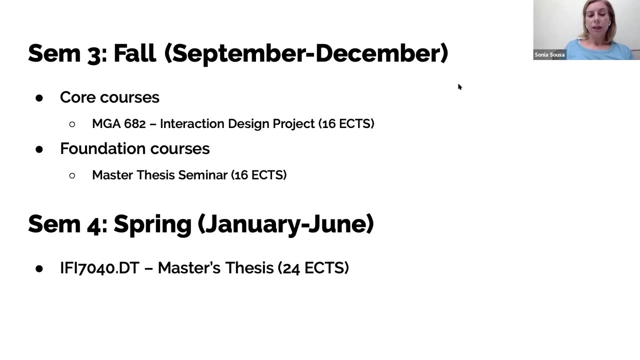 interaction Universal Design. the practice is. it's basically a practice course where you are invited to to practice about the interaction design. on semester three and semester for second year, fall and spring, we have a set of core courses to and the foundation courses in semester three. so the core courses interaction design project, where you put 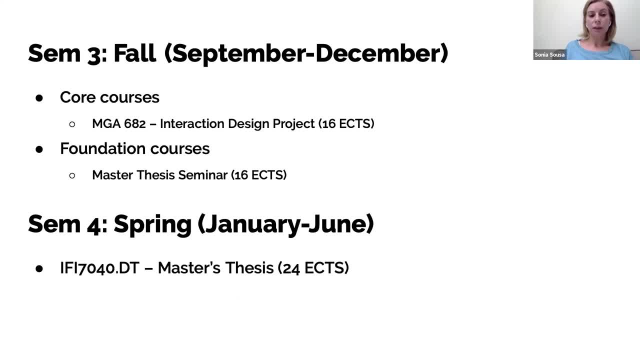 in practice. everything that you learn on the first first year- and the foundation course is your master- is a seminar where you are helped to set up the main research problem and to guide you to, to, to, to, throughout the second, the second, the semester, for that is the master. 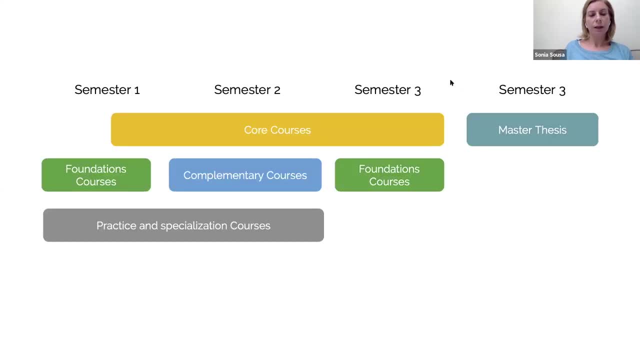 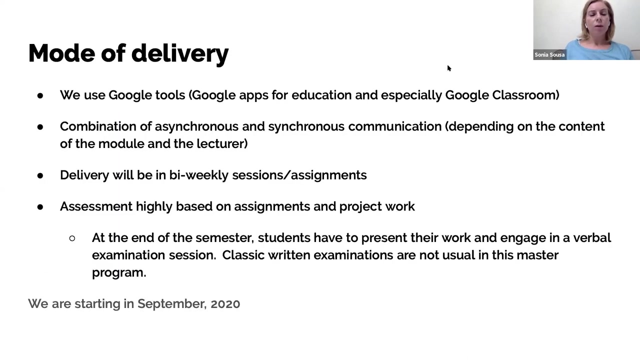 thesis next. so this is more or less what. what it is the distribution of courses throughout the four semester. so we have core courses, master thesis, foundation courses and practice and specialization courses. so for the dreams of future children refers to the development of diverse pathways and I will show you how we can. 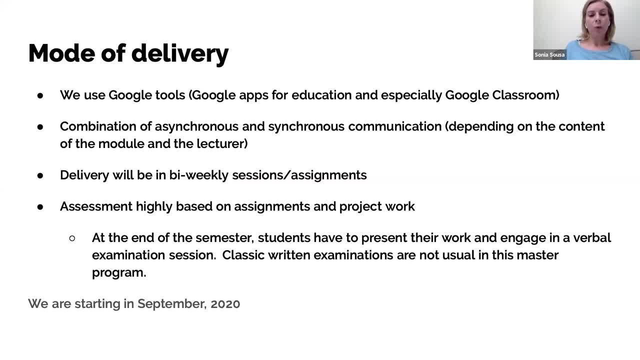 use the birth percent of the course design experience to pergunta to go into more detail about such advanced and system-based mode of delivery available with both the next three of the some themes and structures related to the core course, and another piece to reference is the development of environment. it. we empty ourselves even here, if we, we are half wayfest, discuss how to see each other and a very laughable material based on- hopefully in English, and expressions that may be pretty useful for will it be difficult to understand, which will be used: inkm sonra. 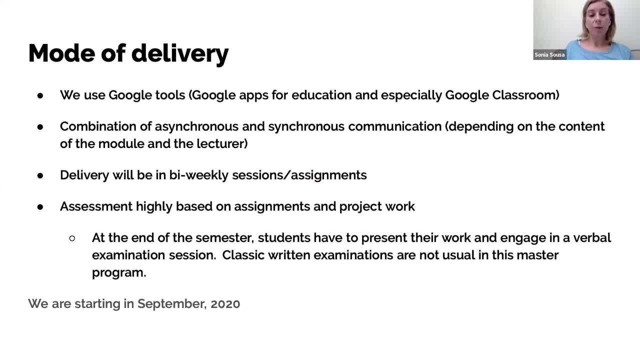 of the assignments and projects are bi-weekly, so you will have a set of assignments every two weeks. The assessment is based highly in the assignments and project work At the end of the semester. we invite you to present verbally in a synchronous session and exam. 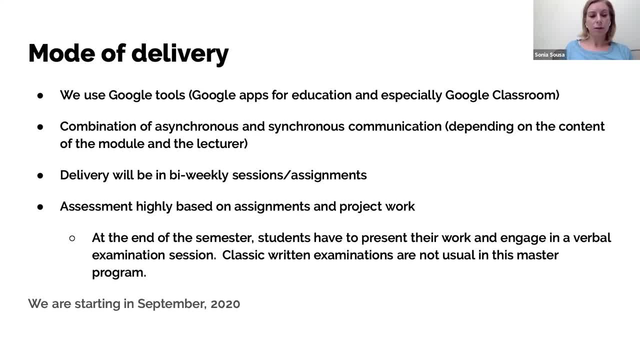 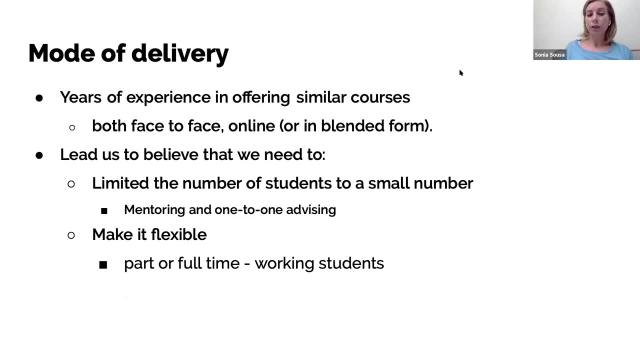 new throughout the course. We are starting this program in September 2020.. So, as I was saying throughout the years of experience in offering this course, both face-to-face and online, we believe that we need to limit the number of students, so this online course- 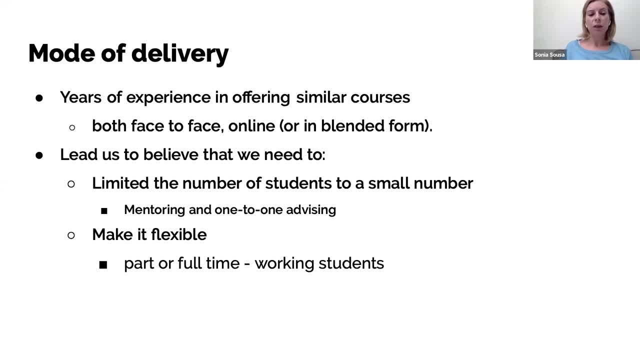 has a small number of students, Because we want to mentor students and do one-to-one advising. We also want to make it flexible, because the main target of students are the ones that are working students. So that's why we offer the course to be run as part-time or full-time, If you do it part-time. 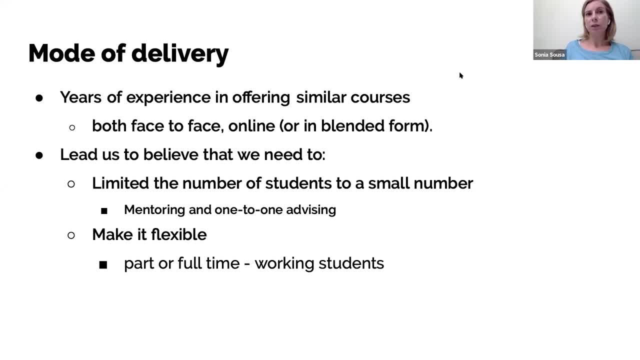 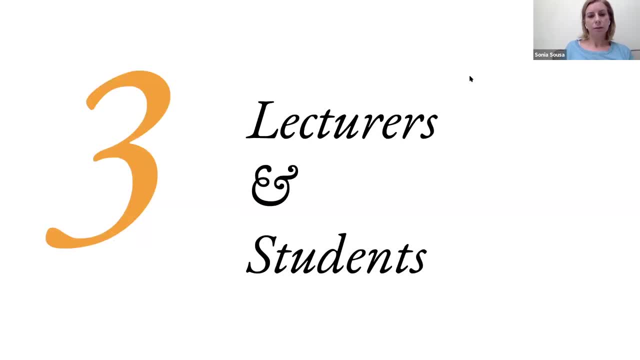 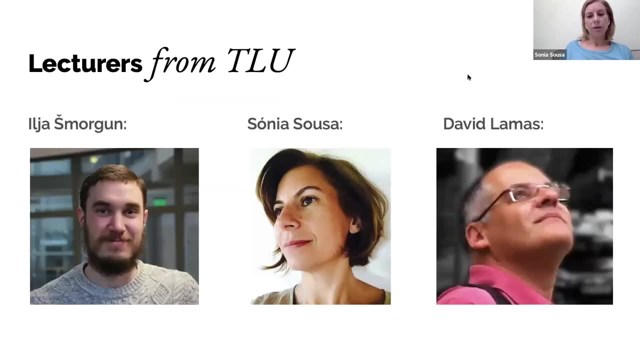 you will do more or less an average of three courses per semester. If you do it full-time, you will do six. If you do it full-time, you will do more or less an average of three courses per semester. Regarding the lectures and the students, So these are the set of lectures for Tallinn. 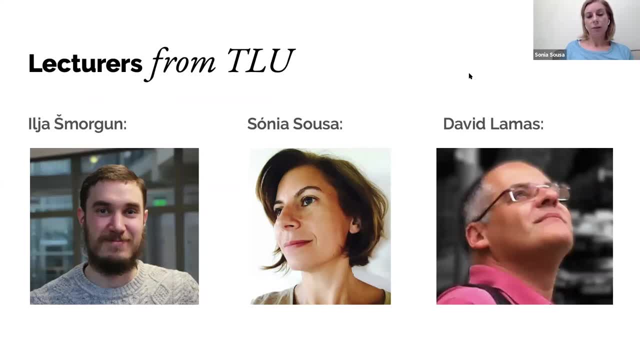 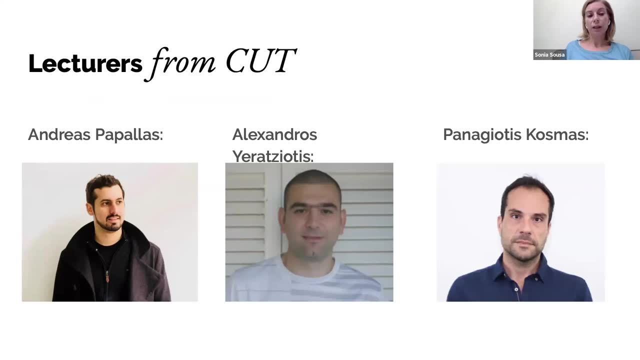 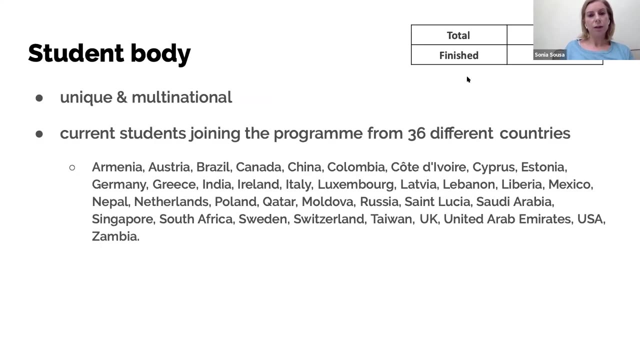 University, Ilia Sonia and David Lamas, And the lectures from the Cyprus University of Technology, Andreas, Alexandros and Panagiotis. Of course we have additional extra support, but these are the main lectures. Regarding the students, we have a unique and multinational 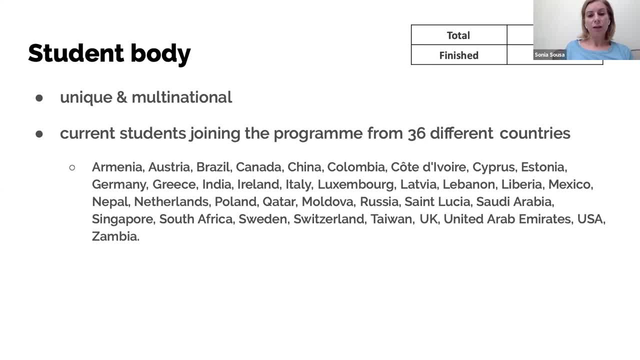 set of students. So we have three students joining us from 36 different countries, And you can see the set of countries here. The total of students that we have right now is 98. And by the end of this year we expect to have 21 students finishing the program. So that's the main lectures. 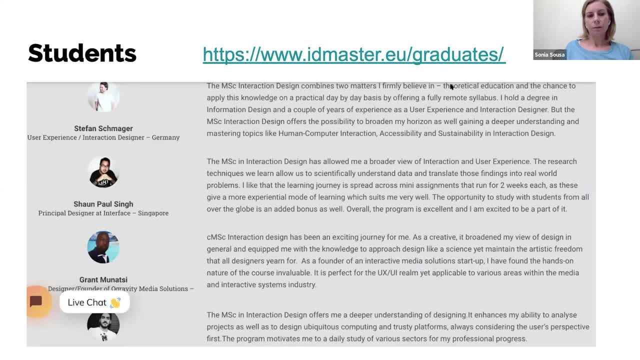 So it's also an additional program for the foreignminists. There are a few lectures that we like to give, but there are buildings which are related tokedocart. Although we know that the teachers are pull out in this year was because I am little late in things. 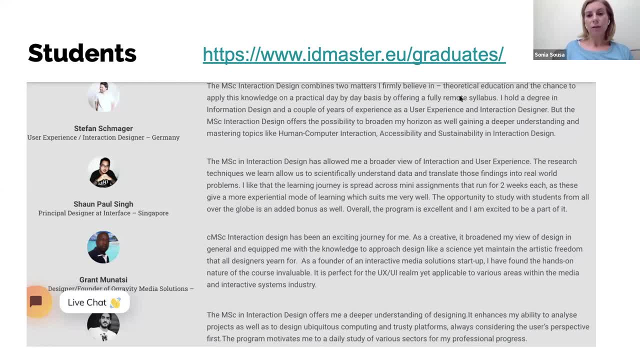 And so by this time will be OK, there is no problem. So if you want to know more about it, you are some testimonials here that you can go and read about it. But Sean will will also be here to kind of present her. he's. we have the problem. Sean, We want you to go and read more about it. You are some testimonials here that you can go and read about it, but Sean will will also be here to kind of present her. he's we have the problem is finishing this semester, so if he has a lot of 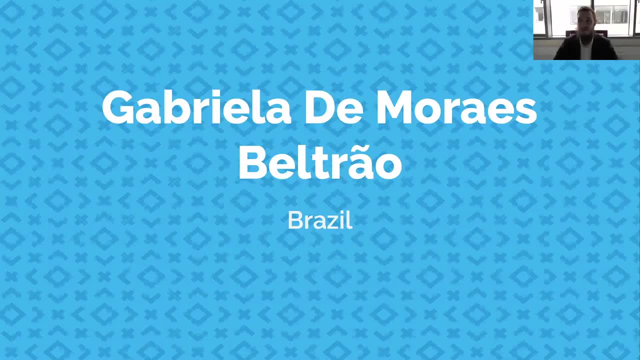 things to say through here, Saying things toorted by Sean. Okay, so that's it from my side, Thank you. Thank you so much, Sonia. So now I'll first invite Gabriela to maybe share some of her experiences. Gabriela is from Brazil originally, but now living in Estonia for almost one year and studying with us in the HCI master's program, So maybe Gabriela can say a couple of words. I think I need to unmute you first. 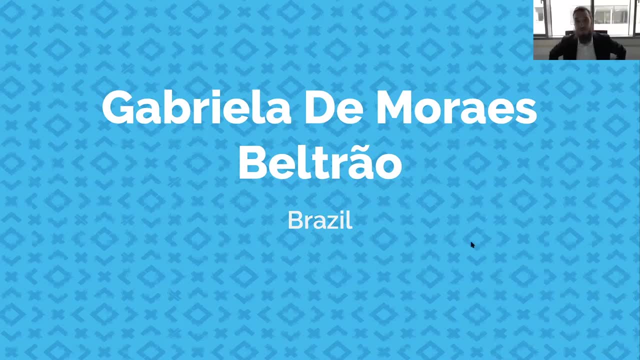 Hello, can you hear me Yep loud and clear? Yeah, So thank you for the introduction, Ilya. So yeah, I'm Gabriela. I'm originally from Brazil. I must admit that at first that was. I thought I would not really fit in the human computer interaction program, because I'm from the from. I have a background in communications. 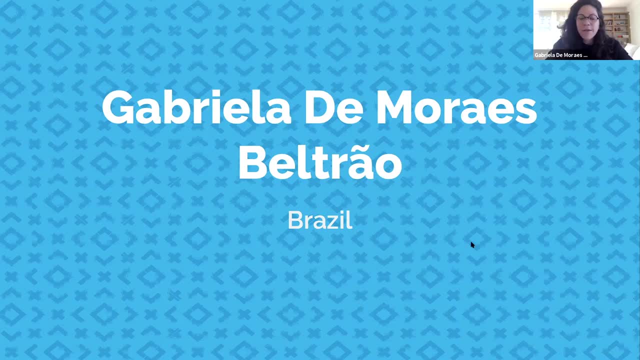 But, as Ilya explained, it's a very interdisciplinary course. It's been really a very nice experience And so far we have a very mixed group. So, the same way that I'm, I'm from communication, I have people from psychology, people from computer science and design, other- yeah, other other- backgrounds, And it's been really good because we can really discuss from different perspectives how how to move on with technology. 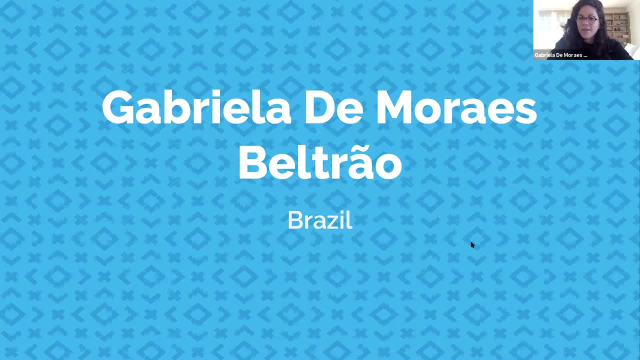 So I think, one of the first things that he mentioned, I think that we, the goal of the program is to create technology for the benefit of people. I think that's really that's really what we discuss here. We have a lot of critical, we develop a lot of critical thinking on on the topic and also have the chance to have some hands on experience. So now I'm I'm finishing the first year, So we are actually still engaged in this integrated project. 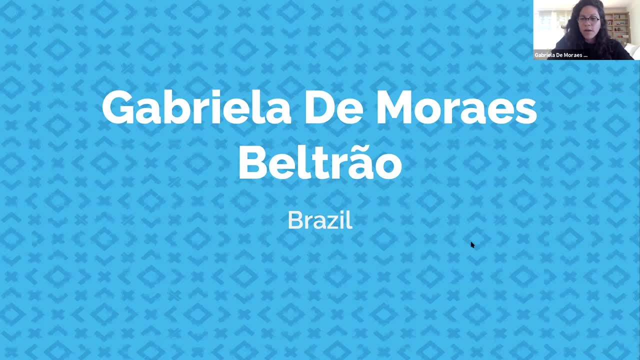 Take back the fantastic Andrei Gyankovitch studies. has been a lot of work really in developing something, So unfortunately we couldn't use all the resources that we have in the lab. Andrei Gyankovitch studies has been a lot of difficulty. all Blo conhecerμο 있고 a lot of amount of ofo keeper en el tixe. a lot ofieważ Security을 relievingnya up by all these efforts. 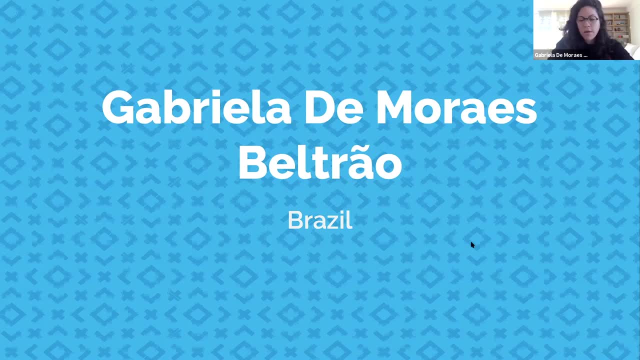 That he also presented me. we had the chance to use some in the previous semester, but but I hope for the better and hopefully as we go along We manage to do everything aligned. but it's nice to know like actually like implementing technology can be really containster to understand the needs of students. 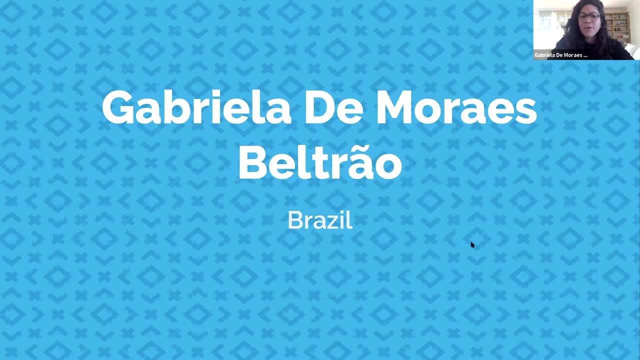 everything it's really there we can really use. I think one of the things that I would like to highlight is that all the teachers from the beginning of the program they're very open to discussions and to really hear what people have to say and helping you out to develop the ideas that you have. 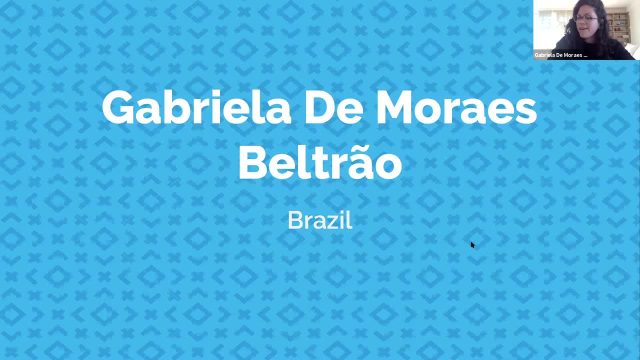 So, yeah, I think it's a good way or it's a very good program, regardless or for different objectives. So I'm really more into this conceptual, I'm interested in this conceptual area of how to make better technology. So I think that's really interesting for me. but I see that also people who are more into developing and creating they also have 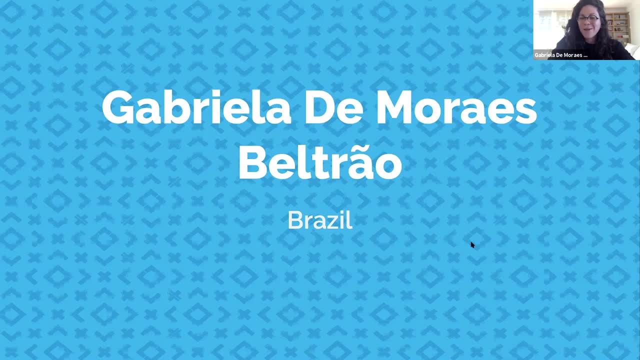 been learning and growing a lot in their practice And, of course, I also managed to develop my skills on that considerably. So yeah, I think that's what I can say so far, Also overall about the university it's been. I mean, it's not a very big university. I think it's a good size. 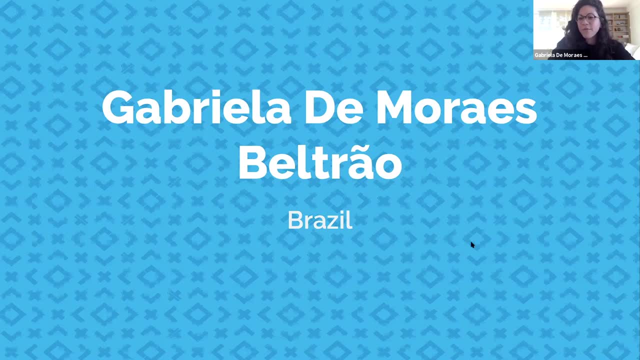 So we have enough space, we have this lab that we can use. It's very, very helpful. It's a place where we can actually make contact with the teachers, with other students from other years, So it's it's very good for the development of our skills. 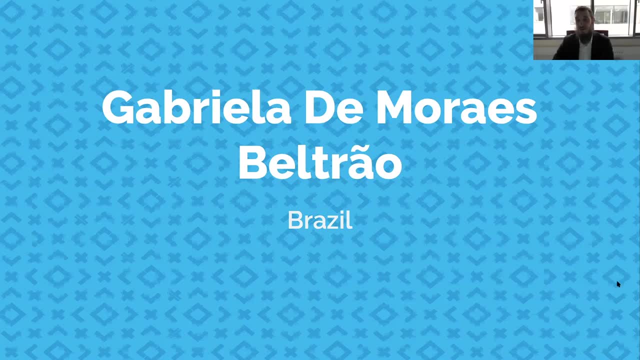 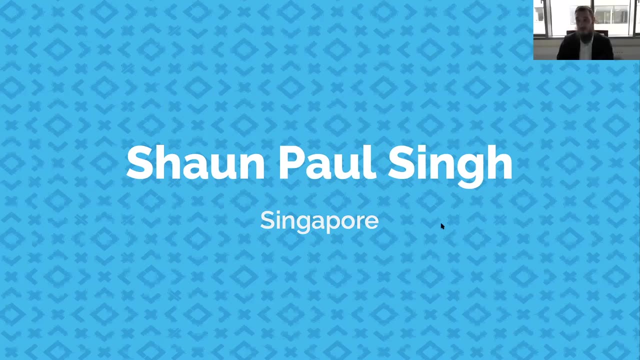 Okay, thank you so much, Gabriela. So now maybe Sean can share some of his experiences in the online masters, please. Okay, hi, everyone from Singapore, So I come from a background in art and computer science, So I'm a dual role: designer, developer. 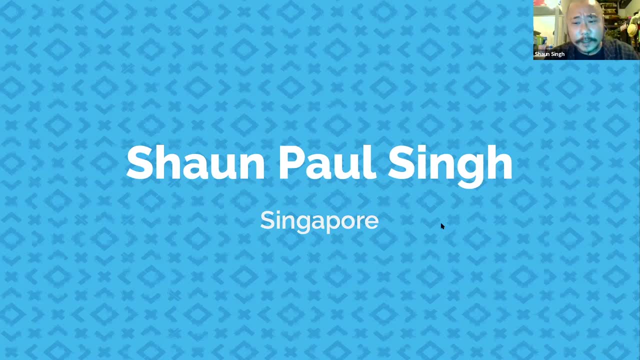 So I guess what made me want to do the program is it would be nice to have a formal grounding in design for computer things. So that's why I did it. I guess most of you guys will be like me, working professionals. So after a while- design principles, everything they get, they become intuitive. 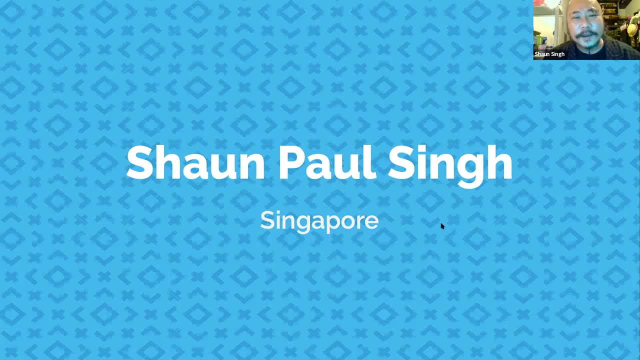 So the whole way the course was delivered. I mean you get it every two weeks, you have an assignment, and it's more or less practical. So it works for me. It is not. It didn't stress me out theoretically that much, which I'm not so good at. 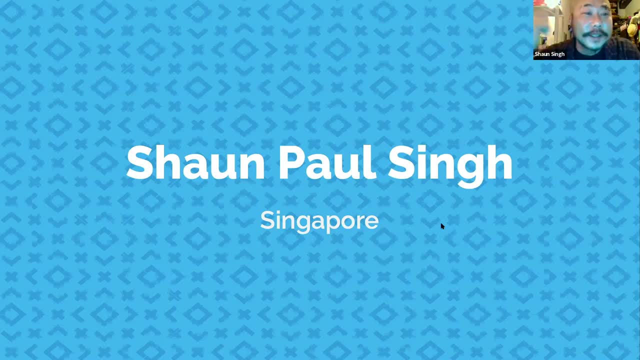 Time-wise. it was great as well, because I'm in Singapore and they are over in Estonia, So the way they deliver asynchronously does work for me. So what I do is I finish work, then I do my assignments, Then we turn in. 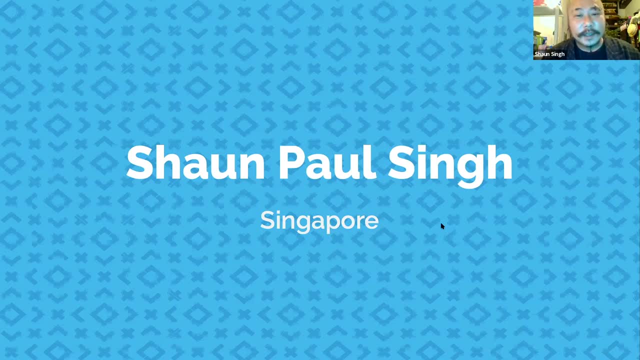 And then we get feedback And then at the end of everything, you do a presentation and then you get the module over and done with. What else can I say? All the lecturers are great. They know what they're doing really. 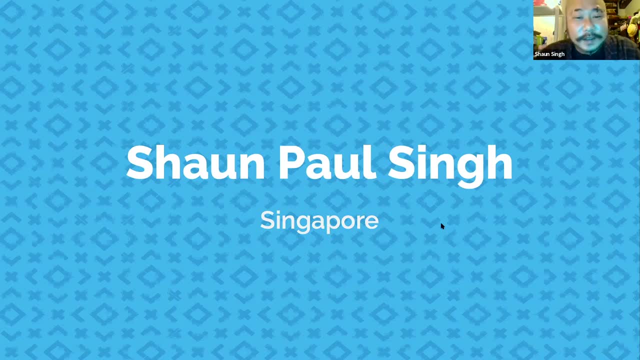 So, yeah, it's fantastic. What else, Maybe, Sean? Maybe he can ask me some questions later on. Yeah, maybe you could mention just briefly your experience with working with colleagues from all over the world. Oh, yeah, yeah, yeah. 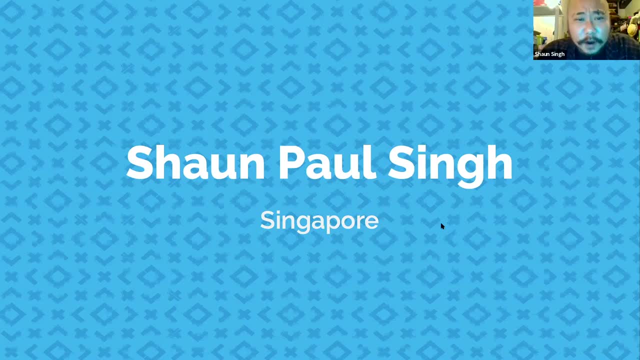 How has that been? It's good. To be honest, a lot of the people you'll be working with are really experienced, So we had Joa, who was already a UX architect. that was like several levels above me, So it's just really inspiring to see him work. 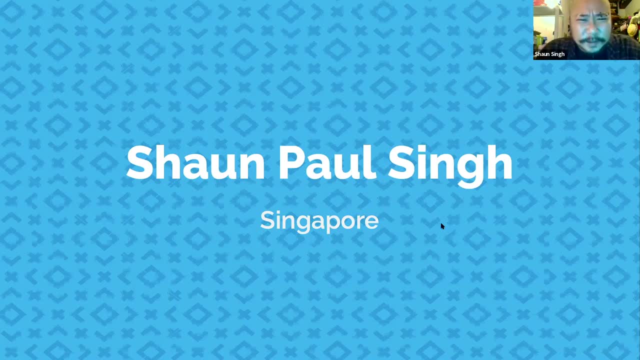 We had Raimunda, who was already senior management, And it's overall quite a good experience. I would say, Yeah, it's great. It's great, I like it. Thank you so much, Sean. So maybe some of our participants will have questions for you later on. 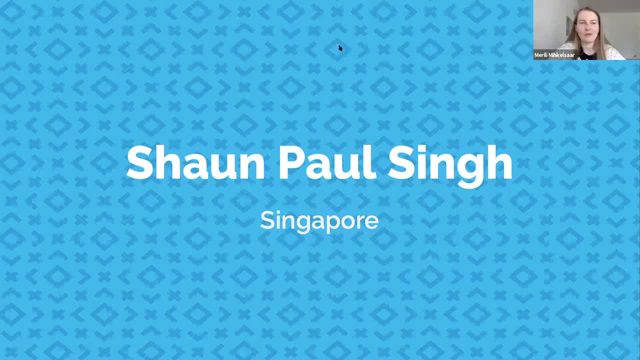 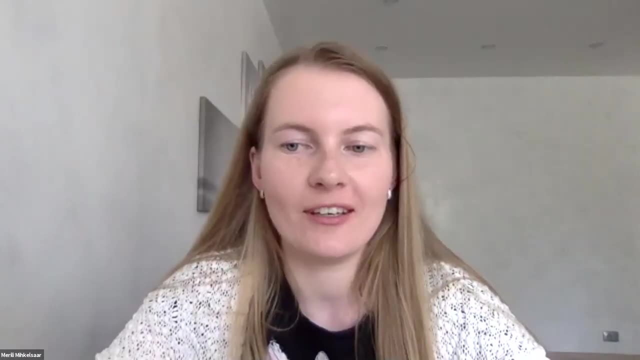 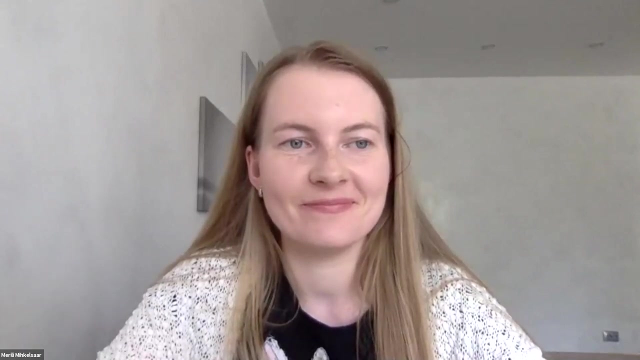 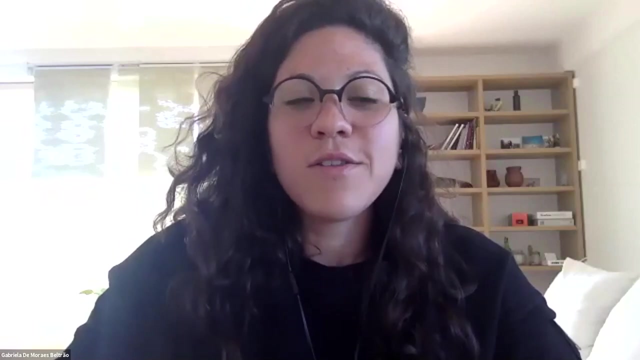 So be ready to answer those. Yeah, sure, We have one more question for Gabriela. Yes, What is your reason for studying And what do you want to achieve with this? Sorry, I was muted So well, I didn't mention before but I'm from communications, but I used to work with advertising. 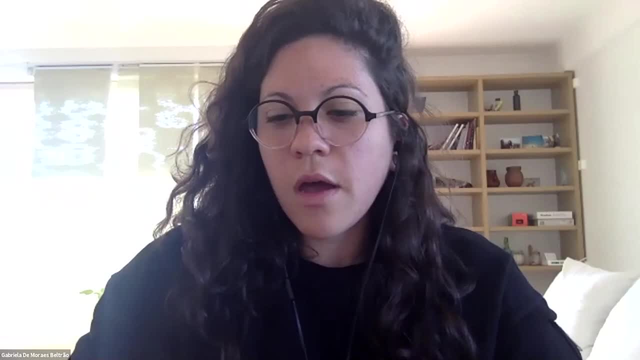 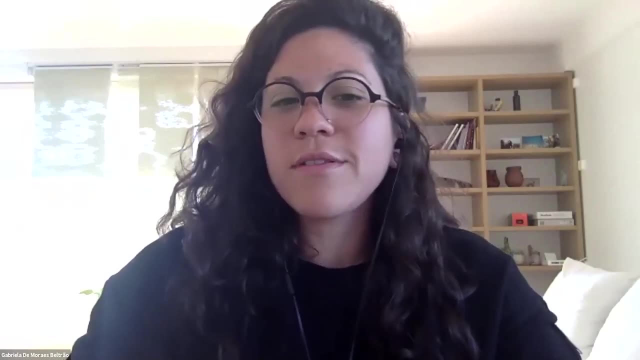 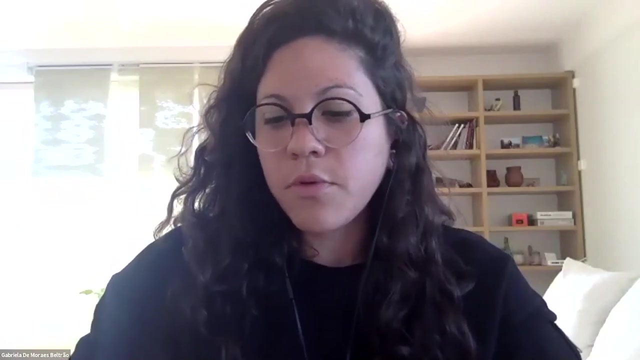 And my initial motivation. it was actually to try to move to the UX field. So in Brazil it's not such a formal field And I wanted to get some formal education that would actually put me closer to that. So that was my initial goal. 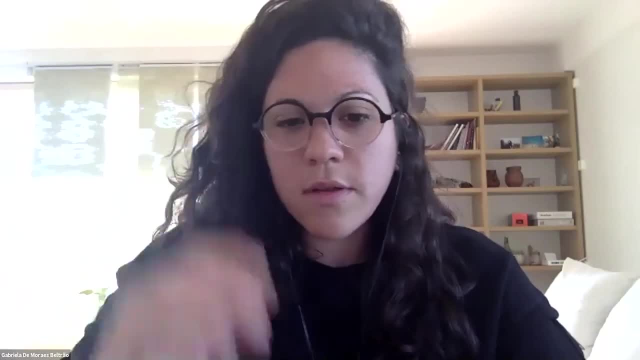 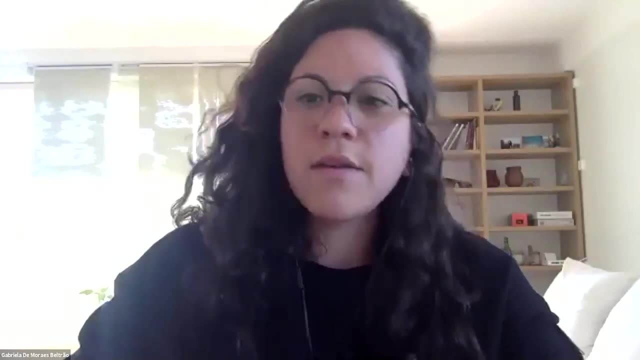 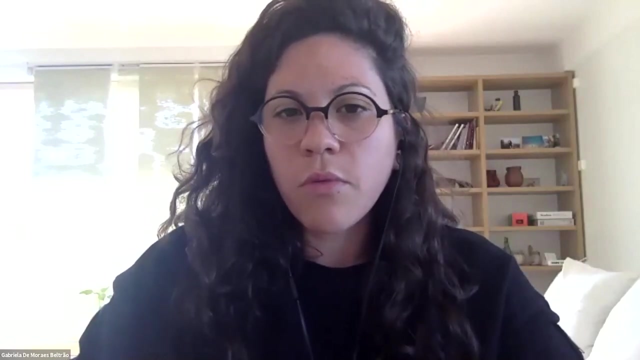 That's why I started. But now I'm really interested in getting more involved into this more theoretical research, And I'm also interested in working with the AI side of human computer interaction. So now I'm considering maybe trying to focus more on research and maybe following a bit further into the academic life. 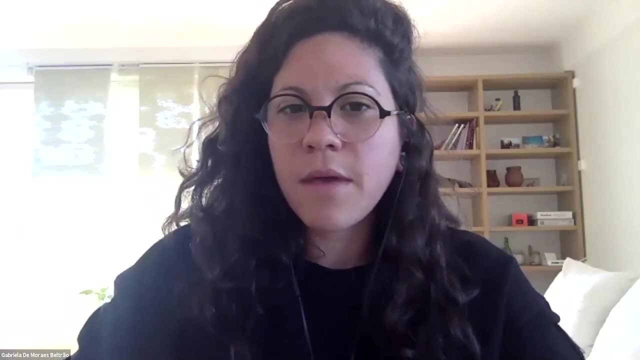 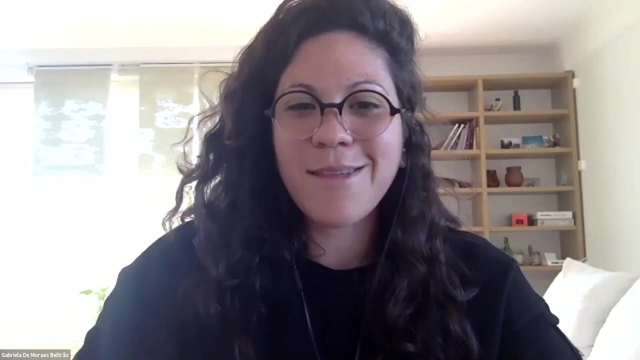 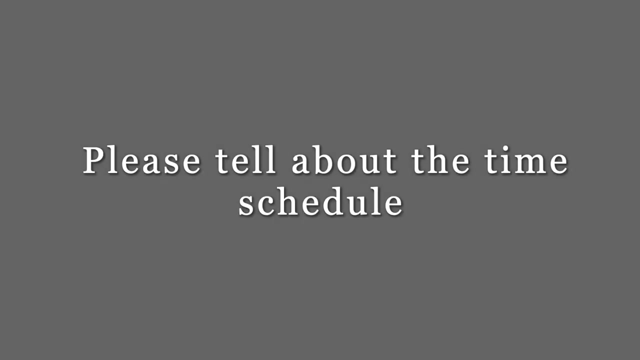 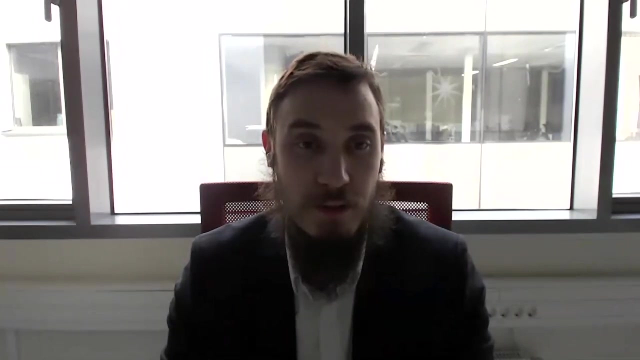 So I'm not sure yet, but I feel like I get I'm getting enough skills to follow both paths if I decide later, So I'm looking forward to that. Sean has already touched upon this. although in the format of the online studies and the face to face studies are similar, 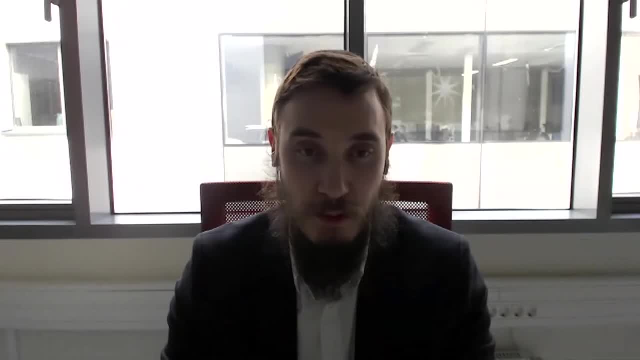 So it's biweekly courses We need every Wednesday, Thursday and Friday. So you need to plan for full days from morning till evening. it's roughly, I guess, 6 hours of classes, 6 to 8 hours depending on how intensive the day will be. 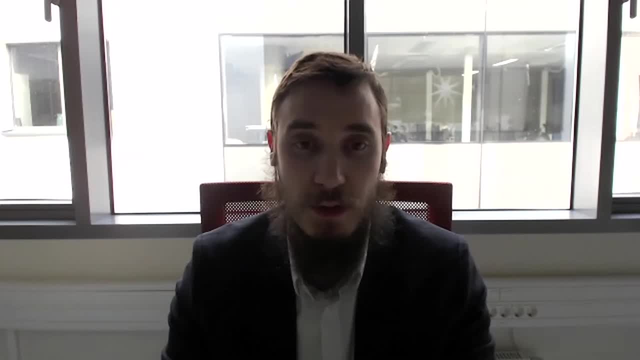 And then you have 2 weeks in between to work on your course. So it's a lot of work assignments, either individually or in group. The labs, as Gabriela mentioned, are open to students 24-7, so usually you can apply for a student pass and then you can go and work in the labs whenever. 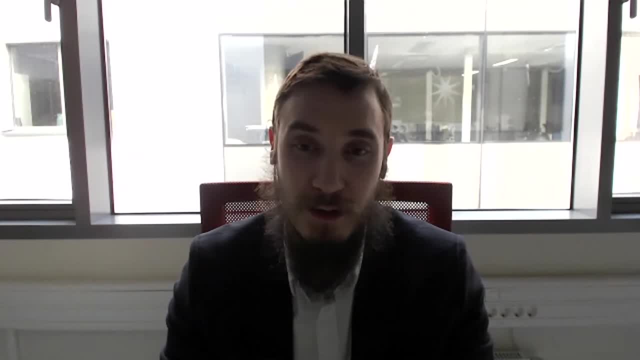 you want to. If you work early morning or late at night or on the weekends, it's totally up to you. Whenever the university is open- it's almost open all the time throughout the year- I think you're welcome to come at your own time, at your own schedule, and work here. 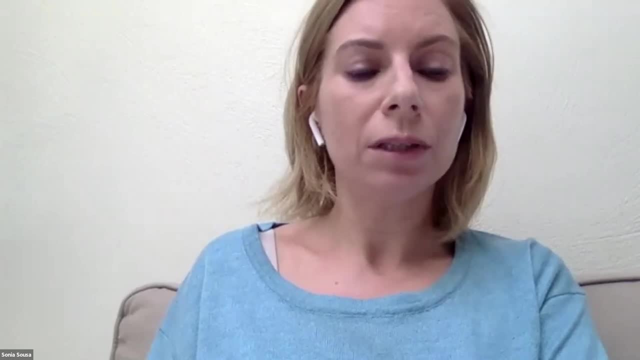 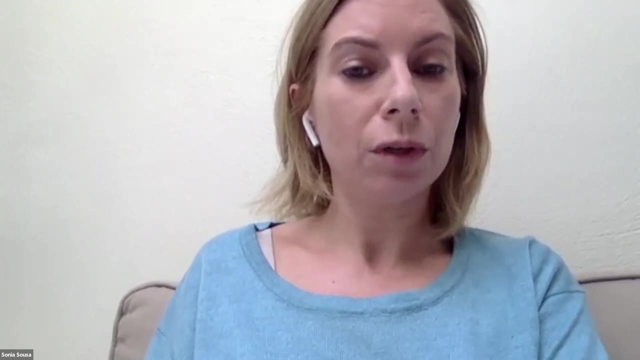 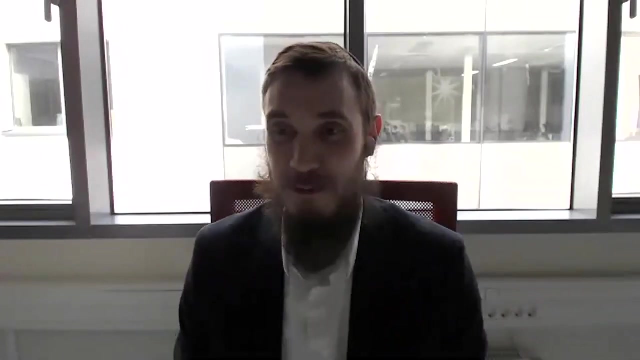 I also wanted to add that in your online course, usually we set the deadline on Tuesdays, so you have the weekend also to work on your assignments, so you expect to deliver something in the end of the day of Tuesdays, Okay, So finally, someone asked the question we have been open, waiting for. what about COVID? 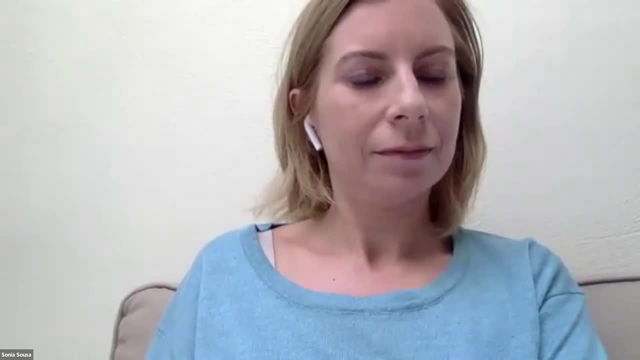 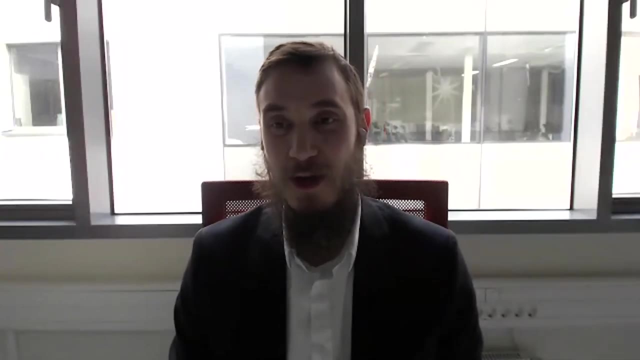 and what do we do about studies in autumn? So the answer is that we don't have an official answer yet. we're actually waiting for that from the studies department, but of course we have been talking about it. For the online masters, it's not a problem because it's all online. 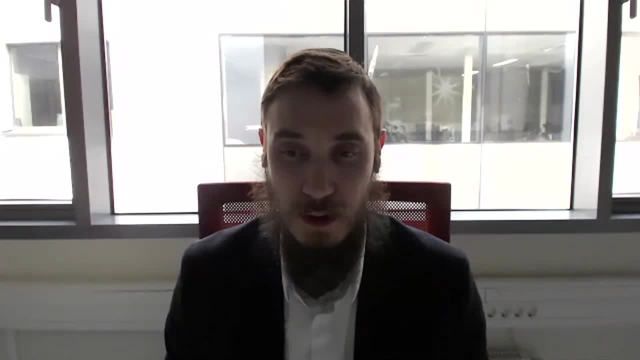 For the face-to-face masters. I think- and this is kind of not the official statement yet, but that's something that we're planning to do at the moment- is to go with blended mode of studies. So those who are able to come here to Estonia for the beginning of the school year are more 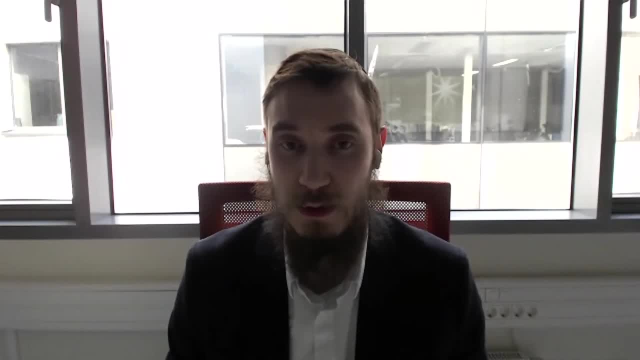 than welcome to come. Hopefully the health situation will be allowing us to actually meet face-to-face- at least there are kind of indications of that- And those of you who, for different reasons, won't be able to come by September will be able to join online in our sessions. so we will have kind of a parallel schedule of online sessions. 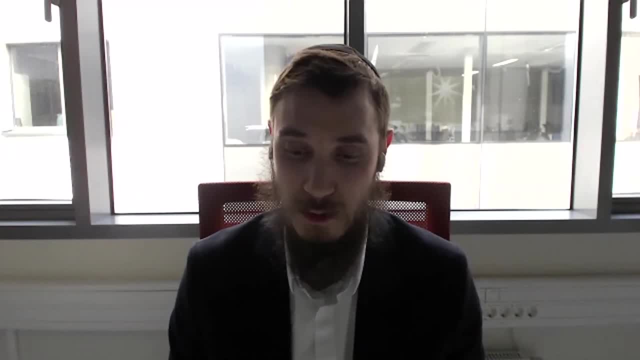 to complement our face-to-face studies, so maybe, in kind of during group work presentations, you'll be joining in online together with our face-to-face students and contributing and participating in that. I guess, like you saw from the presentation of the online masters, we have extensive experience of teaching both face-to-face and online, so it shouldn't be. 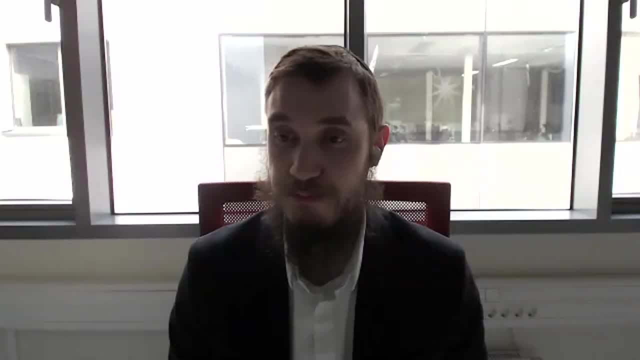 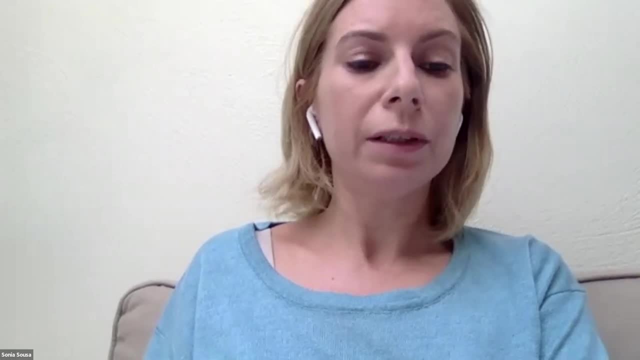 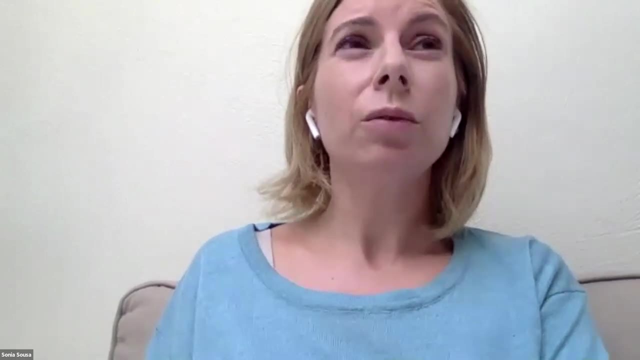 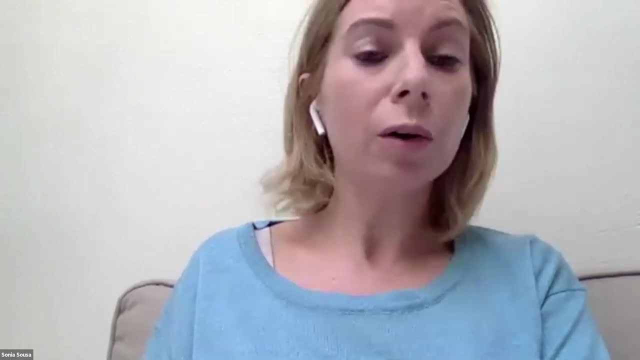 much of an issue of going with this blended mode of studies. It's similar to the HCI, so it's a multidisciplinary program. It's not. we don't demand so high developing and programming skills, so our level of programming on online master is lower than the face-to-face, but the skills are multidisciplinary. 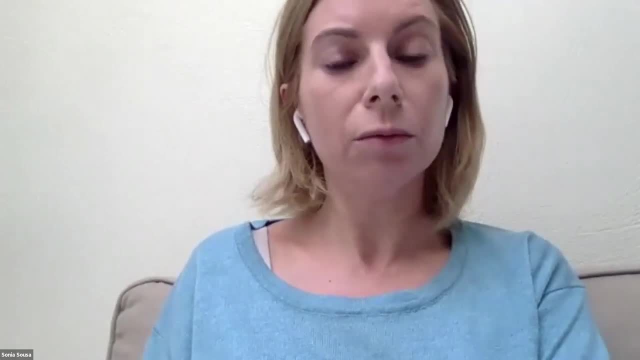 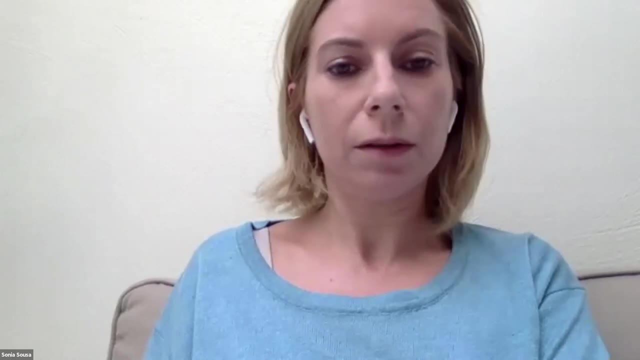 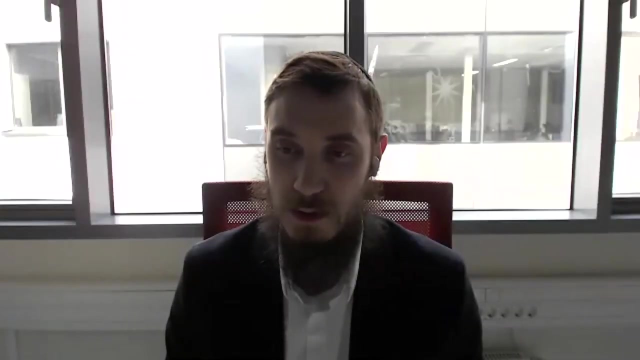 So you can come from different fields and you will work together and you'll share the experience. regarding this, yeah, I hope that I will manage to answer to our question. Yeah, maybe I can just comment on that as well, because the development course was I was teaching. 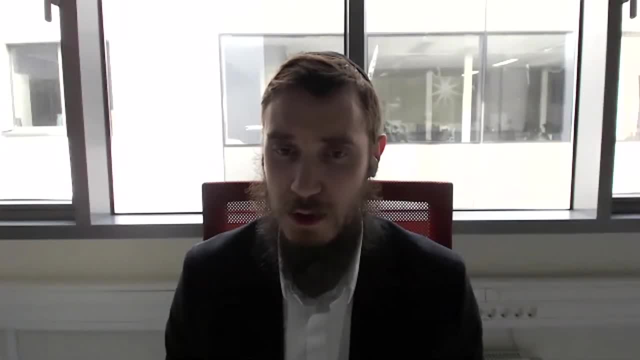 it before. so what we're planning for the new edition is to actually have a full support for you to get you started with the course. Yeah, so we're planning to start with kind of basics of developments and to teach you how to actually put stuff together. So we'll walk you through the process. There will be materials. 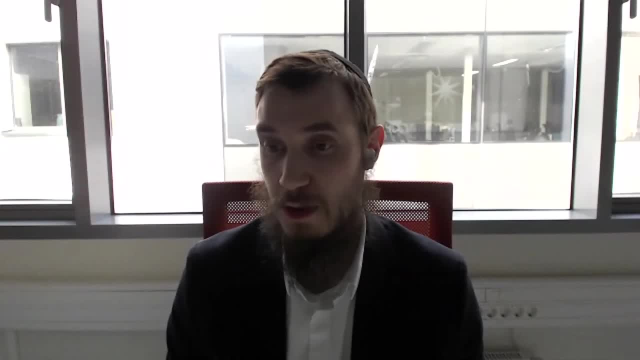 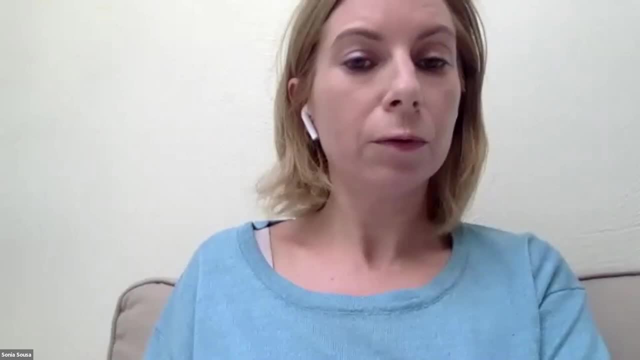 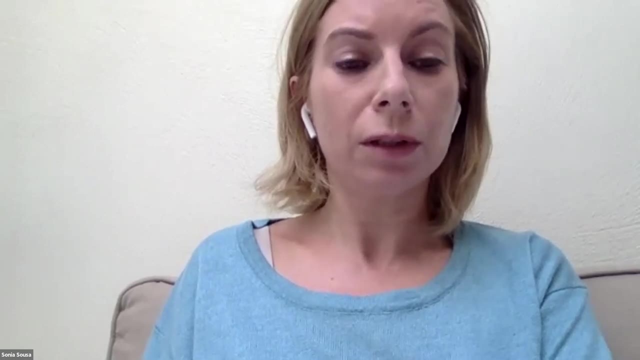 there will be full support so that by the end of the day you can actually make stuff happen even if you don't have the technical skills. So I think it should be quite nice. Of course, we expect to have some technical skills with dealing with all the necessary tools for 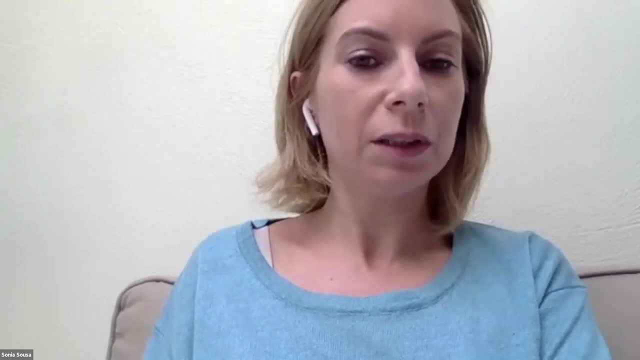 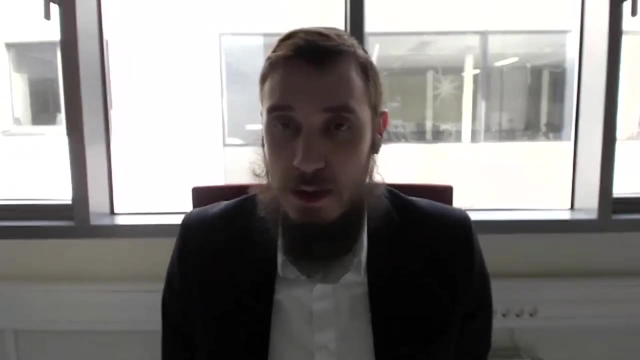 the future, We are probably gonna have to do some development courses for the new edition. Yeah, that's fine. I'm not a computer using the internet, but this is the basic ones. Yeah, yeah, yeah, true, Okay. so Emma is asking about the programming skills for HCI masters. 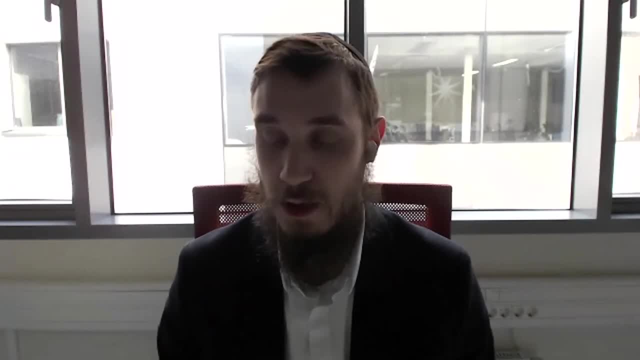 Again- Sonja already touched on it- the background of students is very mixed, It's very multidisciplinary and that's why we also offer this harmonization courses, The harmonization course for, and it fits nicely. it starts in the first semester and fits nicely into the development. 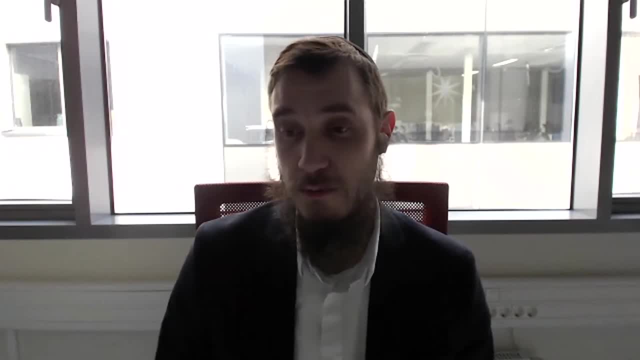 of interactive systems in the second semester. so you'll go from the full range of kind of really basics of programming to putting more complex stuff together, like android applications, eventually also getting introduced to to arduino and microcontroller. so you'll get the full support. so the only thing that we ask from you is kind of motivation and interest to get started with this. 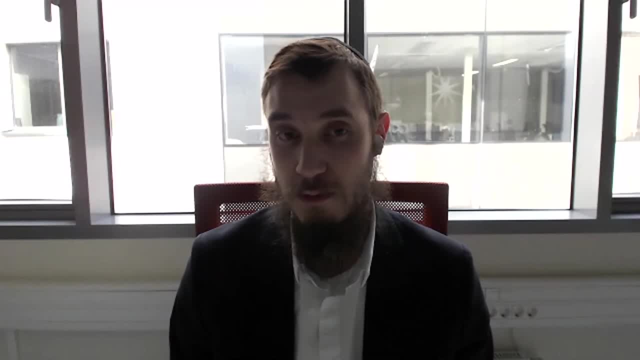 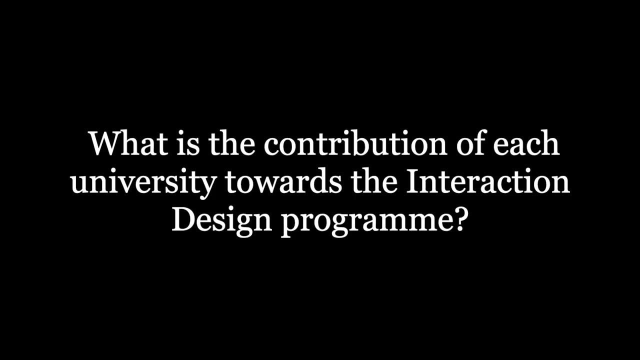 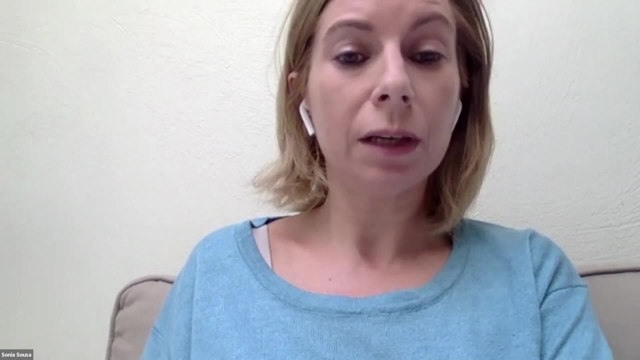 even if you don't have the, the background being open and being willing to learn new stuff, and then we'll kind of walk you through the whole process. so so it's, it's mainly off off. we have a little in italian university, we have a bit more credits, so we we 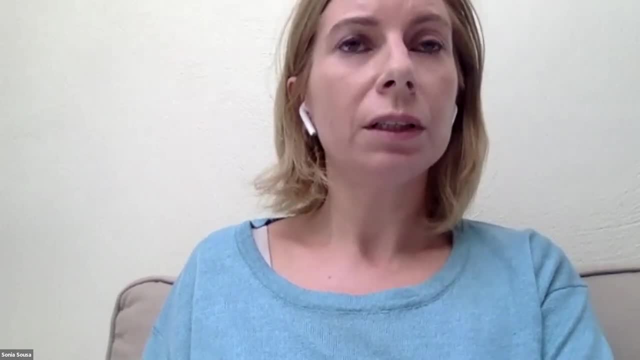 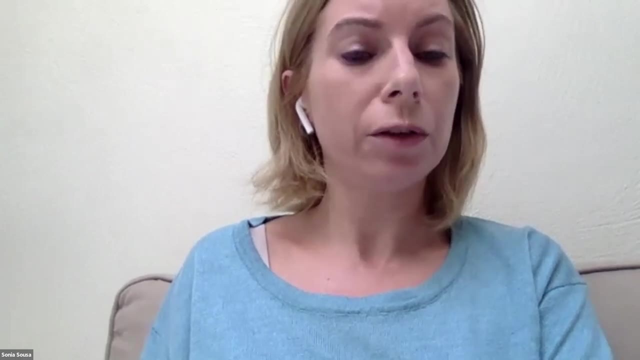 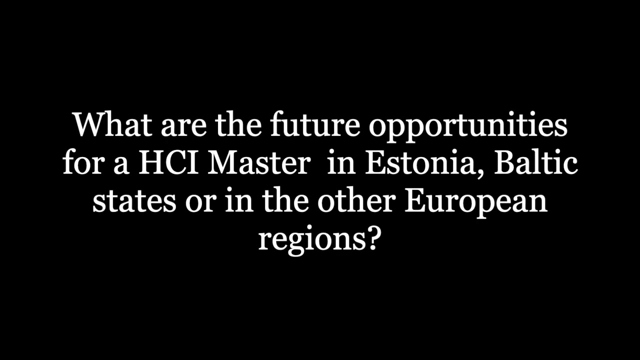 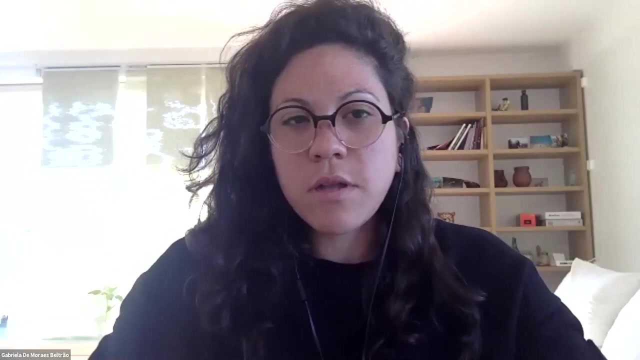 we run. it's a program that it's 51 percent from italian university and 50 percent from cyprus university of technology, so it's one percent more from italian university. so well, so far i've been. i chose to dedicate only two studies now, but several of our class 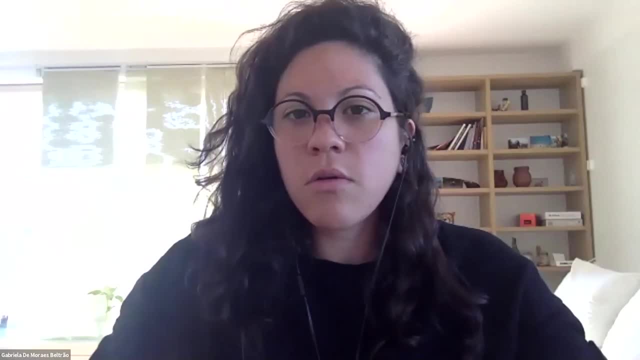 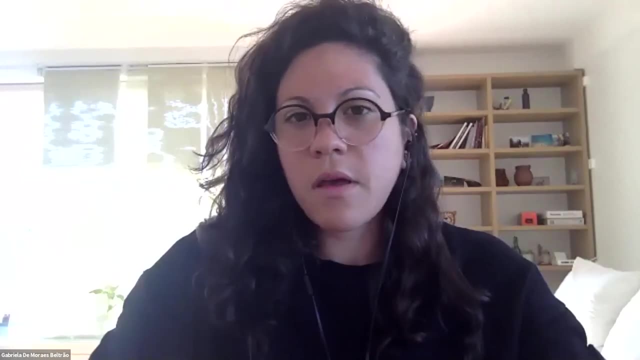 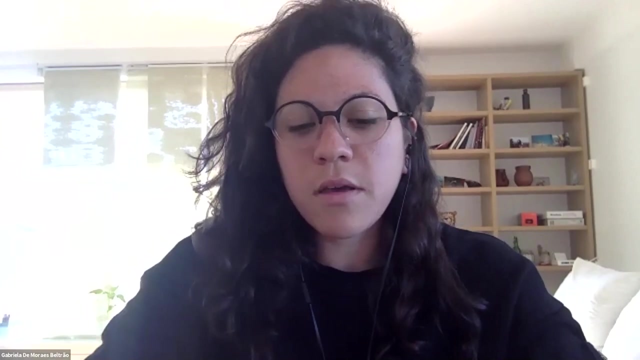 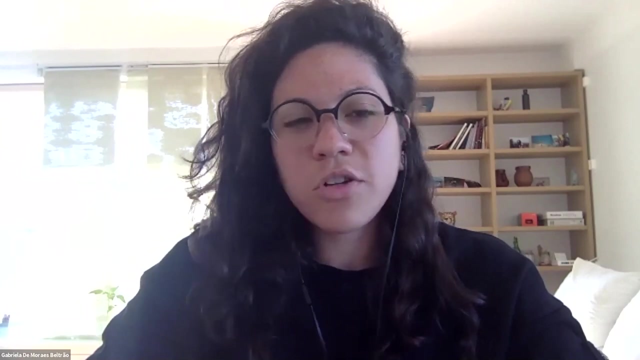 of my classmates. are you already working or already found something? so there are several, several startups and companies and in estonia. i haven't really researched much in the other baltic countries, but they i believe that it's quite similar, i think, overall in this hci field. 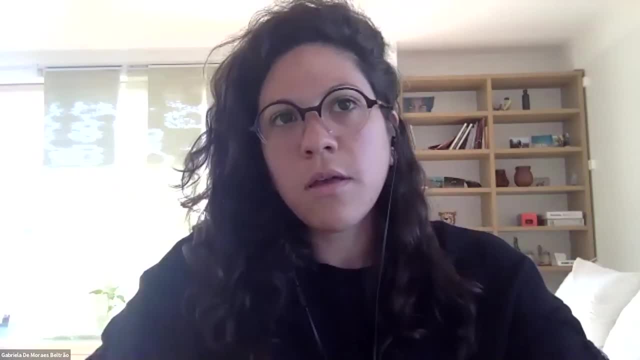 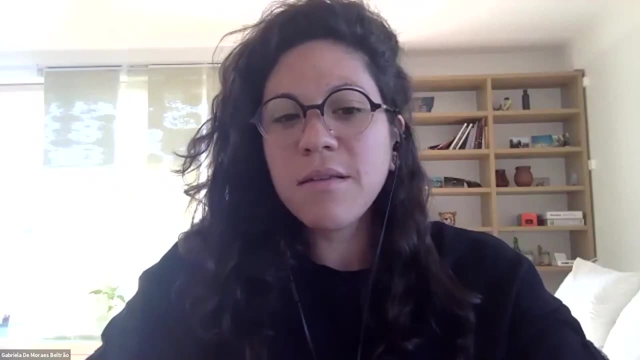 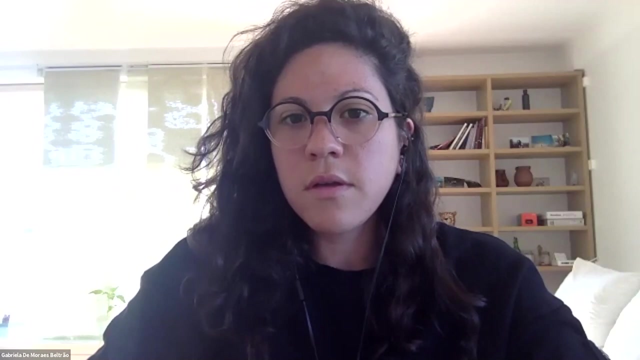 either for more to the side of programming and computer science and also for the side, for the side of design. there's quite a good demand. i would say there's, there's people needed, like skilled people needed in this regard. so it's i. i foresee good opportunities there. there are. 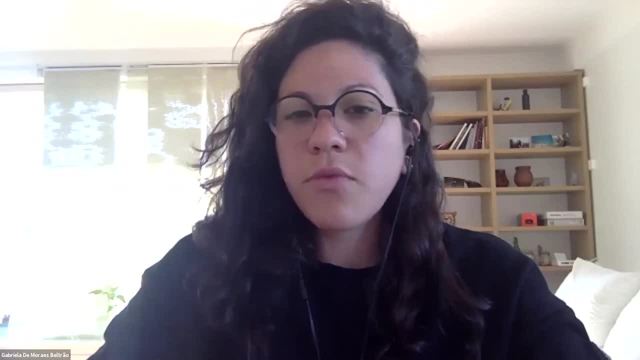 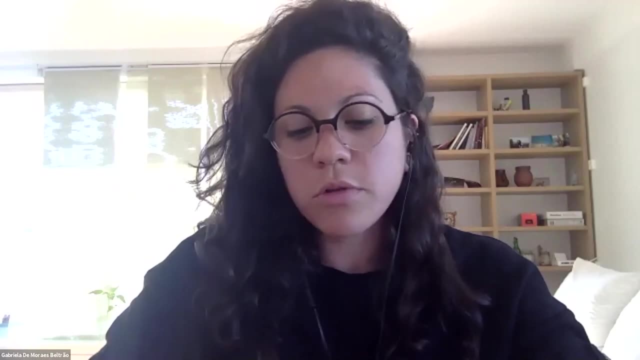 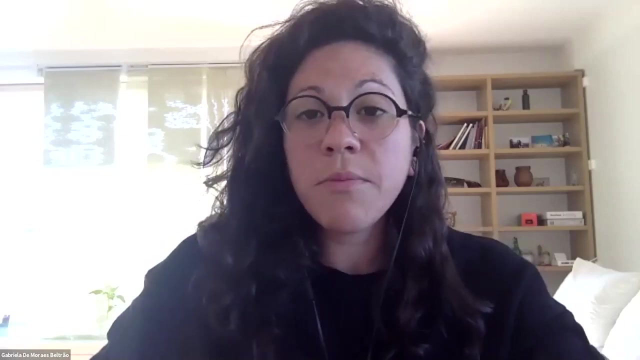 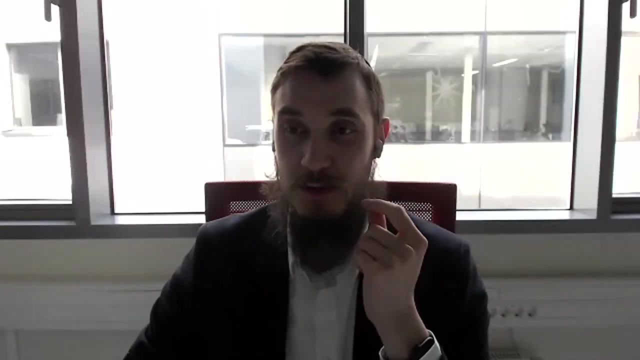 possibilities to work there also, even within the university. sometimes we we get contacted about opportunities for for work or for projects. so uh, yeah, overall, i would say there it's promising field here. yeah, and it's also a challenge for us teaching stuff, because our students i um go start working um either by the end of first semester or by the end of the first year. 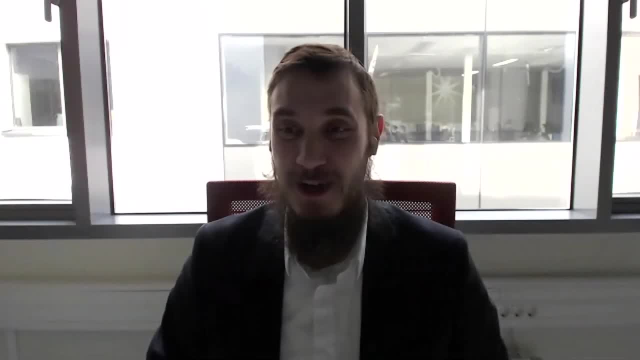 and then we need to chase them. so it's a challenge. we're kind of happy that they can find a job, but also not not happy when they get distracted with the job and not focusing on their studies. so that's kind of it's. it's um, it's kind of two sides to the to the coin, so but i would say in general, 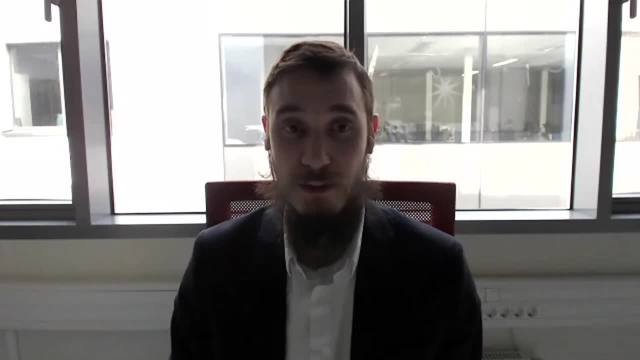 there are good opportunities in estonia. maybe not immediately in the first semester, but as you start getting some hands-on skills, then experience shows that by the end of the first academic year most of the students can get a job, maybe on a slightly lower level initially, but then gradually progressing to higher levels um to eventually some of our alumni. 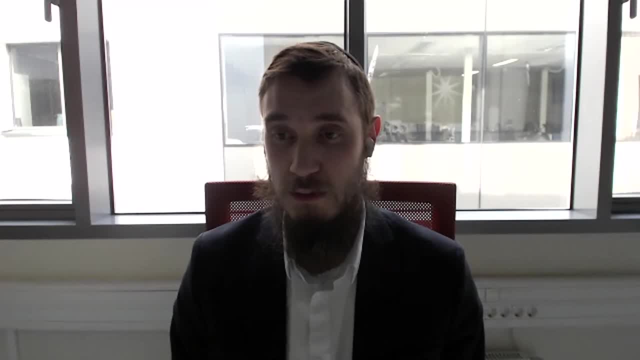 having very nice positions, uh in the in the uh it it sector in estonia. so most of them are done, working it's, and then it's, like abril said, it's your decision whether you want to kind of not work deliberately because you want to focus on your studies or you want to combine somehow. so 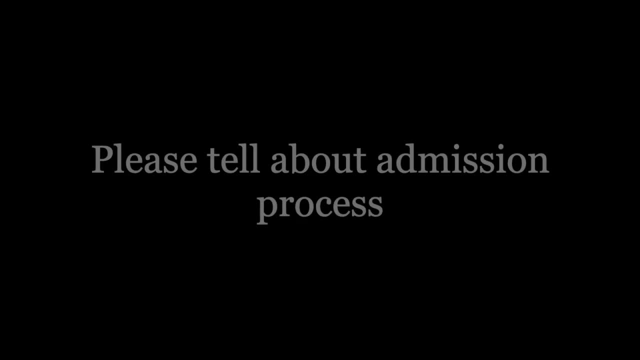 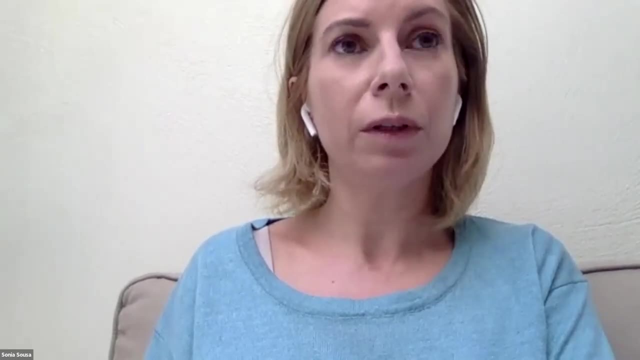 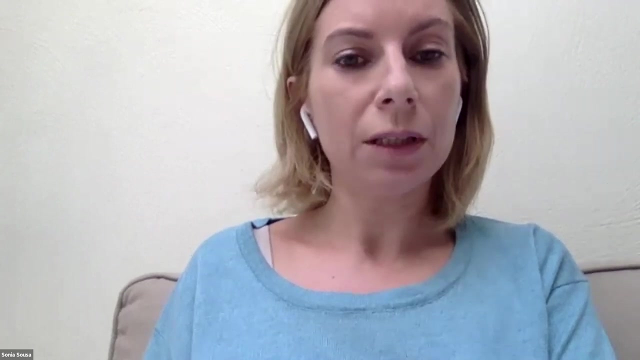 there's, i think there are good opportunities. eventually, we have two types, two types of admissions. we have a documentation admissions, where we go throughout all the documents that you submit and we assess you in base of the documents and then we do an intervention, an interview admission. so this is the test that, uh, maybe we're talking about. 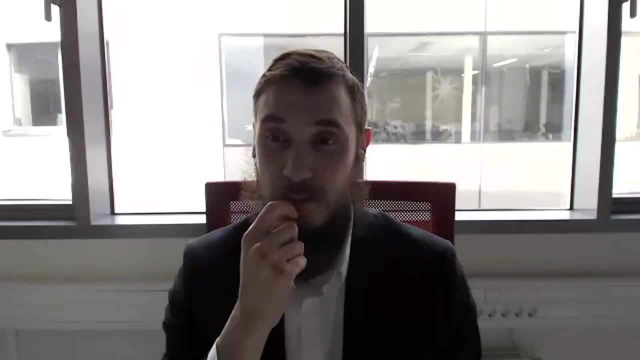 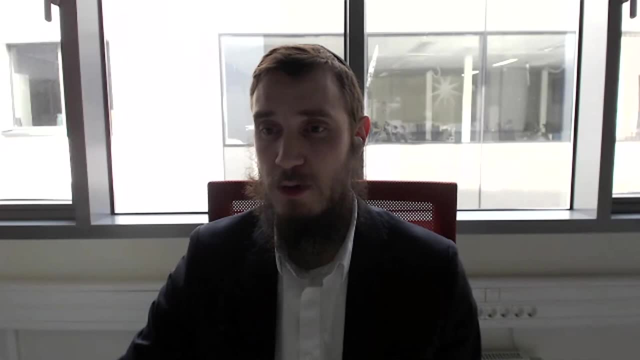 uh, ilia is, isn't it? from a hci point of view, yeah, so there's a, there's a process that you need to submit. it's it's your cv motivation letter and presentation letter, and then you need to submit it, and then you need to submit it, and then you need to submit the application letter and portfolio, and 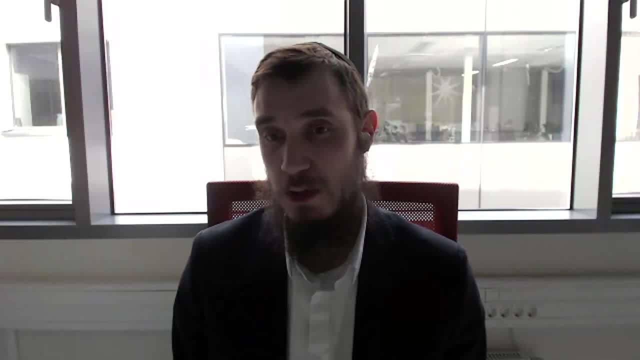 then we in the admissions interview, um, we spent half an hour per each candidate uh, actually meeting you um online, uh synchronously, and then we're gonna go over your um interests, uh, we ask you about um eventually, the the topic that you would like to work on for your master thesis. 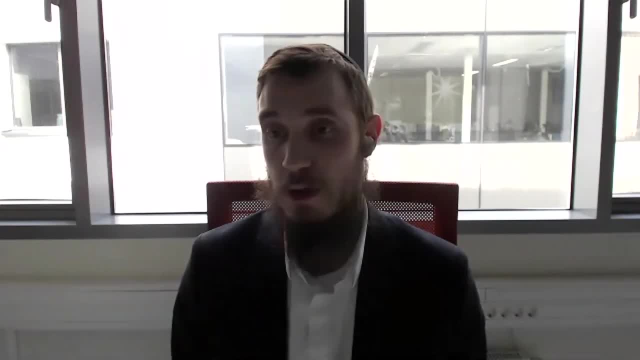 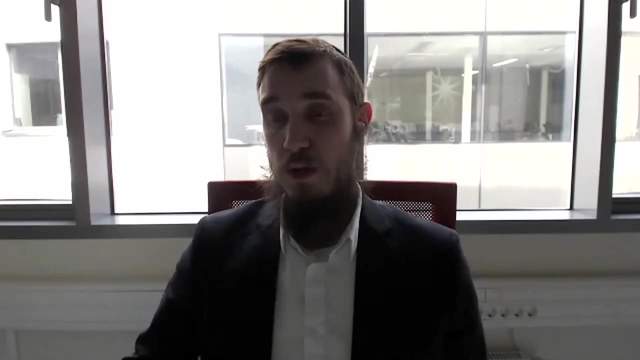 um your skill set, um some projects that you have worked on in the past. um, and, yeah, we try to assess, kind of, and your motivations for the future. so that's that's basically what the admissions is all about. well, um, for designers, we really go um very deep into the methodology and theory of design. 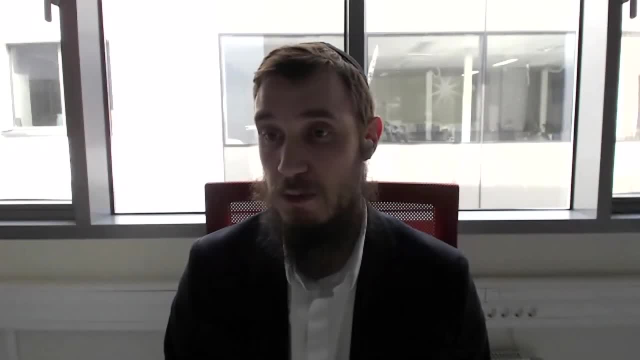 uh, the different theoretical frameworks, um, how to systematically approach the design process, um, and of course, also the technical side of things. so if you're lacking the technical skills, then we would, of course, expect you to invest more into learning the basics of programming, how to put stuff together so that, uh, eventually this integrated project that gabriella mentioned. 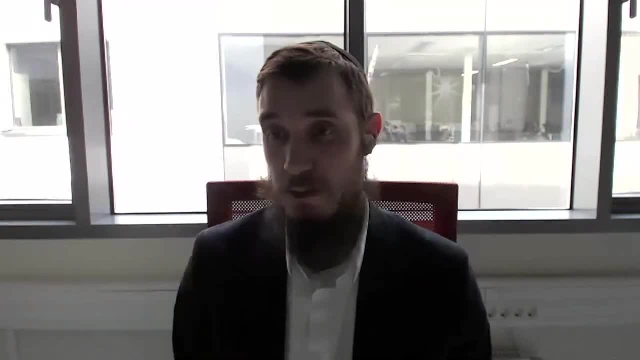 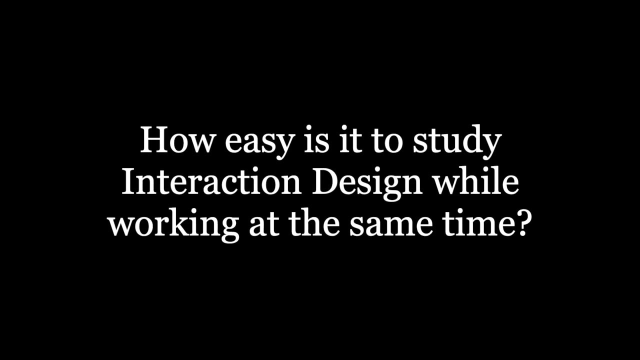 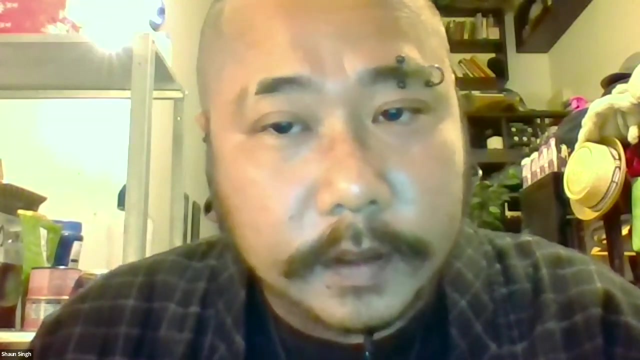 that she's now working on with her colleagues. um, in the second semester in spring, you would be ready to actually actively contribute to, to building stuff, um, so that's that's kind of the learning curve that uh us designers would go through. um, what i did was i was studying full-time and i took the program full-time as well. 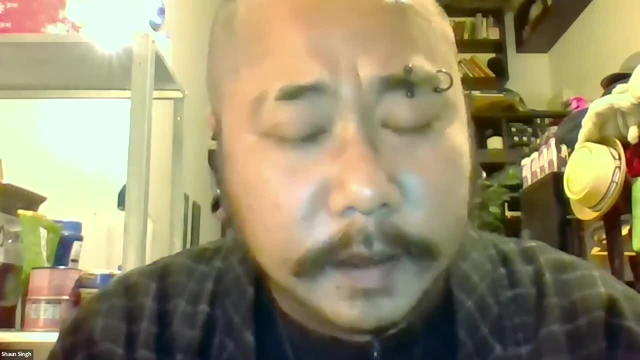 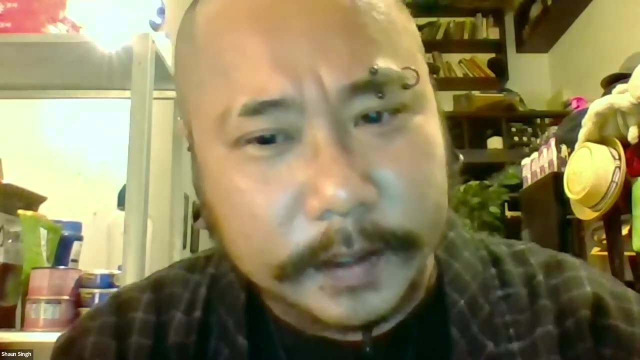 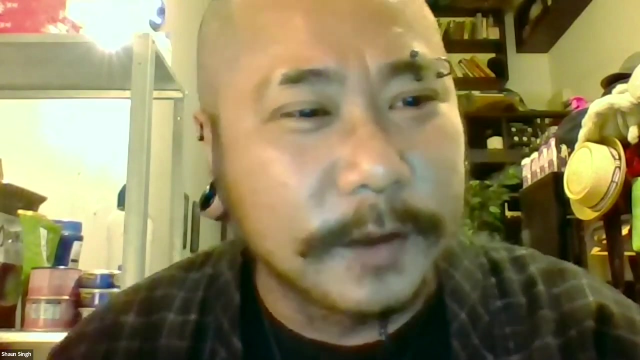 so it definitely can be done, but i think what most of the other students did is that they took three modules and then they they worked at the same time. so, um, it's really up to you to judge how how much load you can handle, i guess, but it can be done, i. 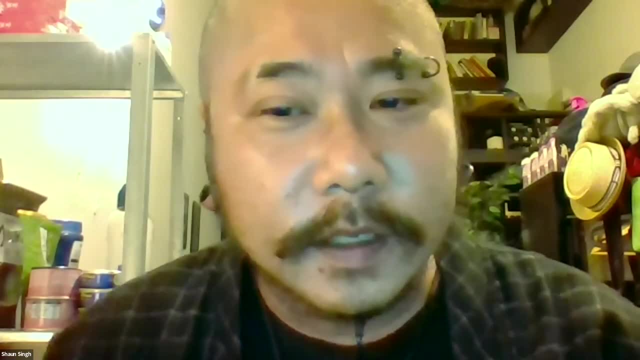 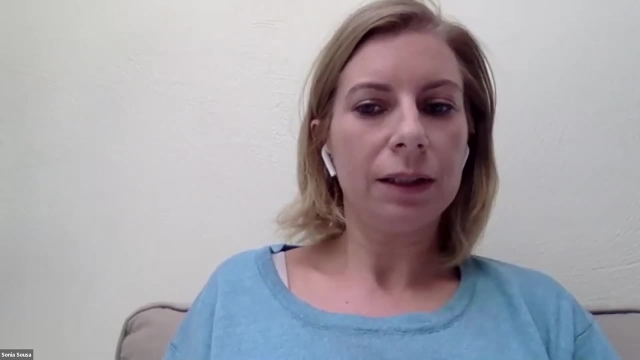 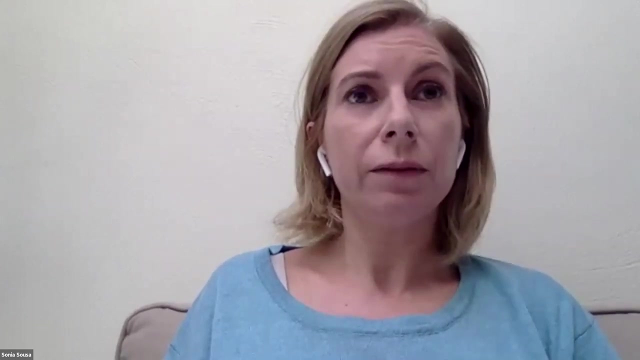 did full-time work and i did full-time studies, so hope that answers your question. we also advise students to to try and see how much courses they can handle they. they can start with three enrolling three courses and then, if they feel that they they can handle a little bit more than then, the next. 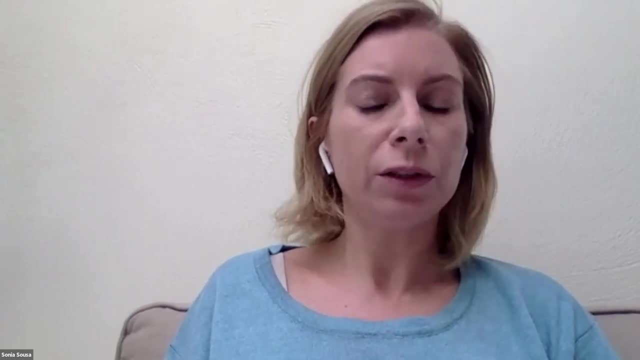 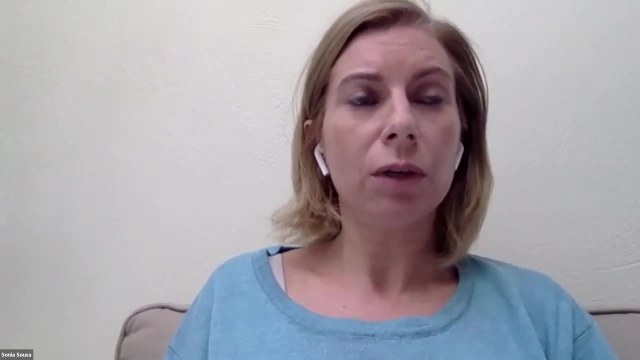 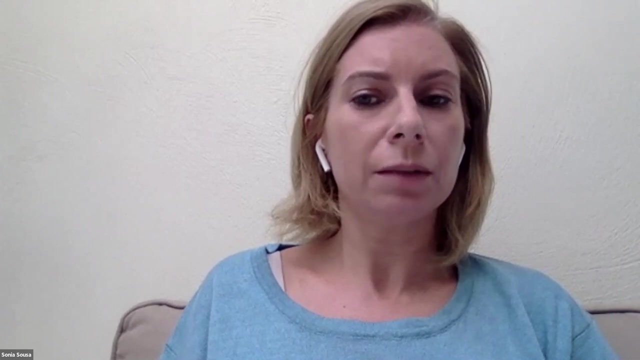 semester. they can enroll in four or six, it depends on them the same. the other way also works. so if, if you feel that, uh, you cannot manage the the workload, then you cannot let us know and you can reduce the amount of courses that we enroll in the next semesters. 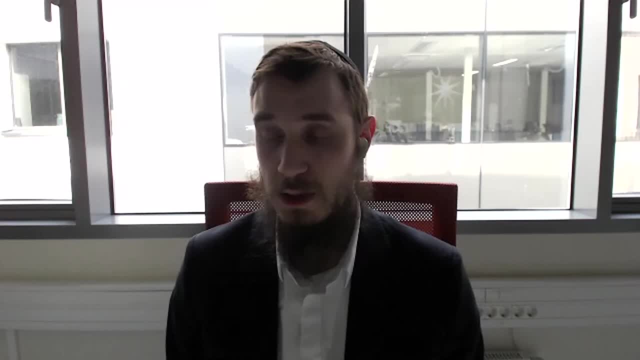 the courses are mainly full semester, um based in hci, although in some cases we have intensive courses for lasting for one or two weeks, but these are mainly exceptions. normally the courses last for 14 weeks- that's the length of the semester, but which means that we will have 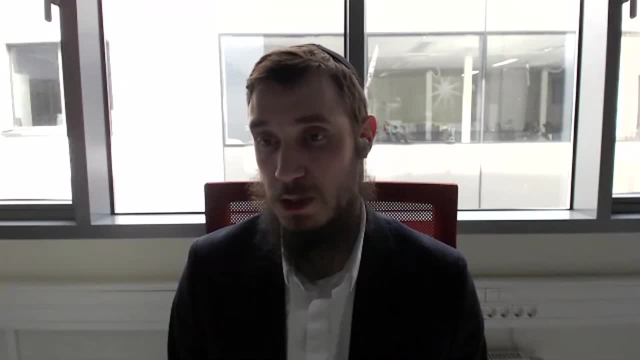 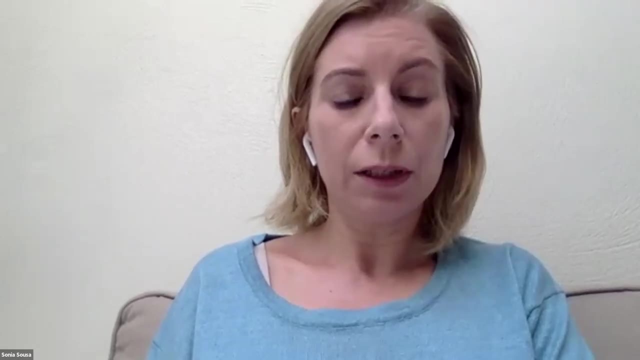 an average of seven to eight contact sessions, so one session every two weeks. so this is the average schedule for the courses. to clarify as well that for the, the online master in interaction design, you don't need to submit a portfolio. you can, but it's not obligatory. so, for those who were,